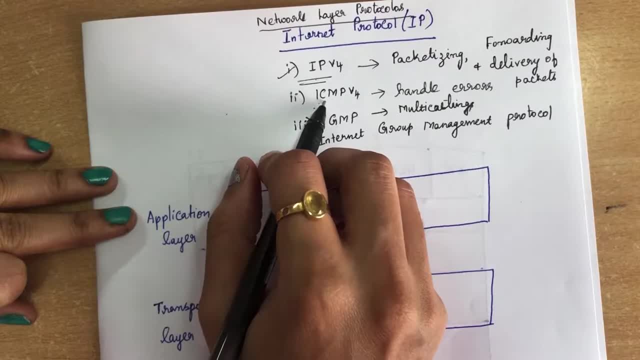 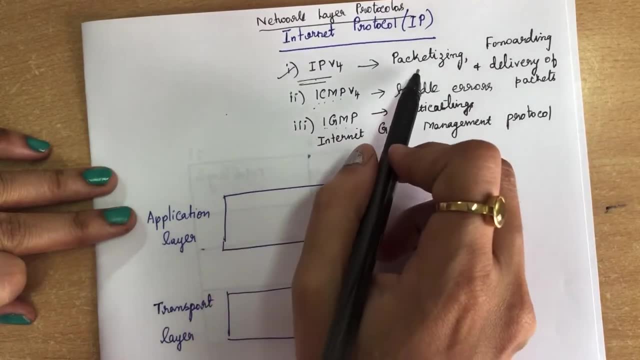 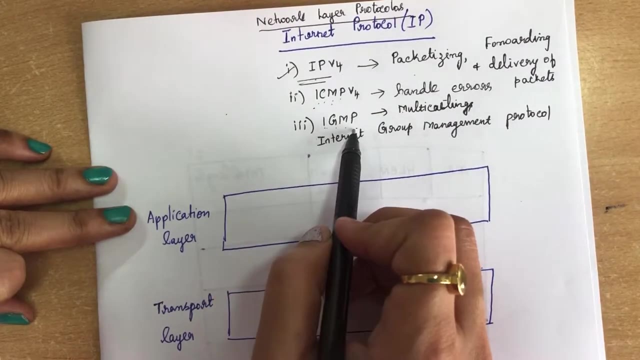 is internet protocol. Second is ICMP, internet control message protocol, Then the third one is internet group management protocol. This IP protocol helps in packetizing, forwarding and delivery of packets. ICMP protocol will handle the errors and ignob protocol will help in multicasting. Okay, so first we will see the position of internet protocol. 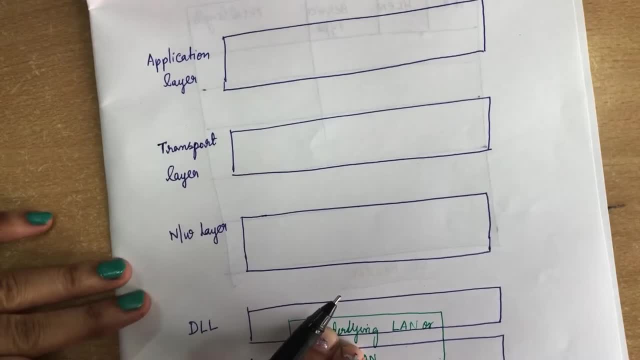 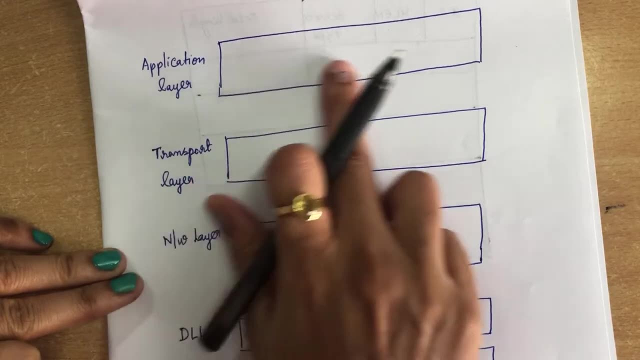 and other network layer protocols in TCP IP protocols. So in TCP IP we have a physical layer, datalink layer, network layer, transport layer and application layer. So we will see what all the protocols and which has been placed in this, all these layers coming to application layer. 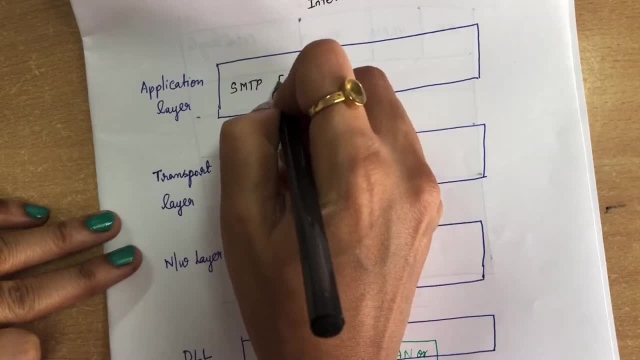 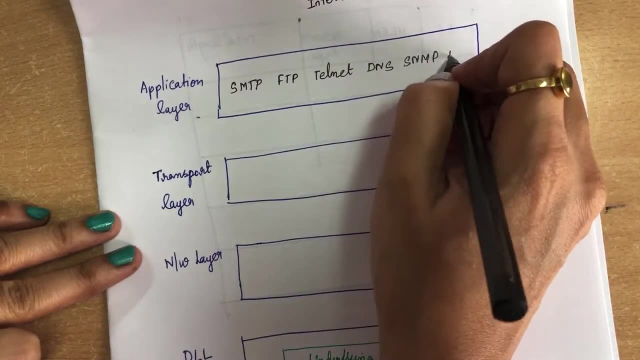 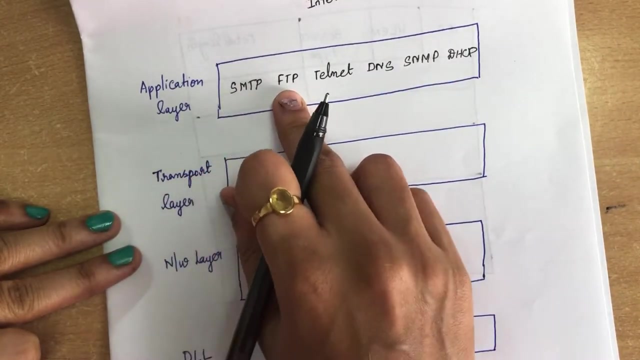 so it has several protocol that is like smtp, ftp, telnet, dns, snmp and dhcp. okay, these all several protocols which will be studying in application layer. smtp is simple mail transfer protocol. ftp is file transfer protocol. telnet domain name system. dns is domain name system. snmp is simple. network management protocol and dhcp is dynamic host configuration protocol. next, transport layer contains tcp and udp, that is, transfer transport control protocol and user datagram protocol. next, coming to the network layer, network layer as these protocol, that is, igmp, igmp and icmp placed in the top and internet protocol placed in the middle, and you have 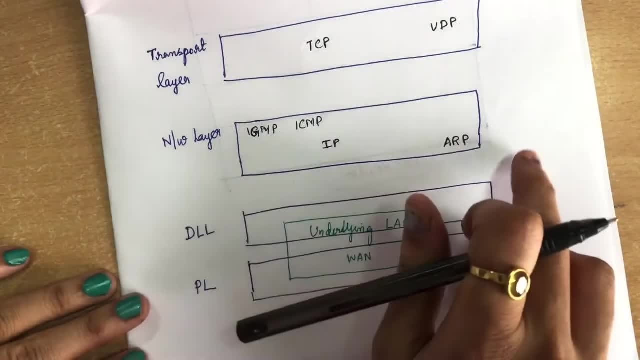 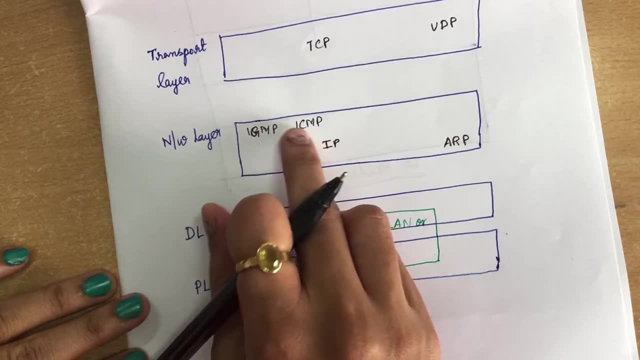 arp protocol, which is placed in the bottom of the right side of your network layer. okay, so igmp and icmp, it is placed in the top. that is internet control message protocol and internet group management protocol and control message protocol, and this is ip protocol and arp is. 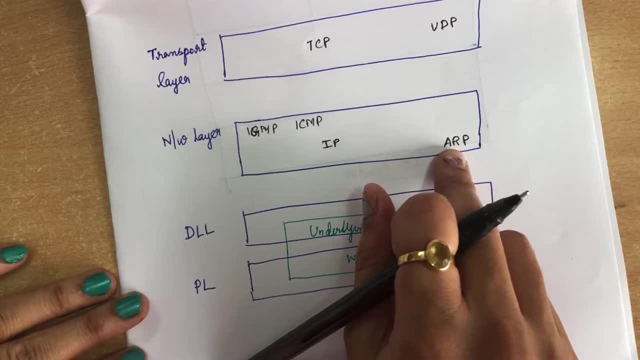 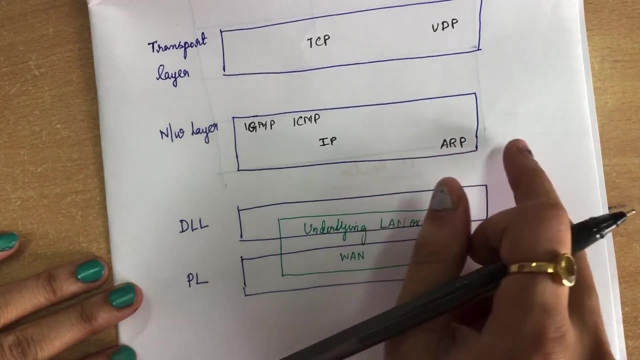 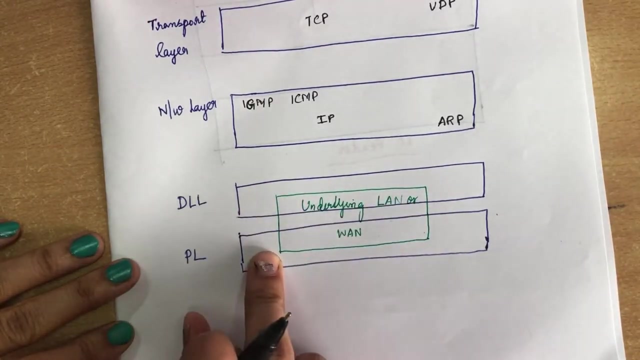 address resolution protocol. this already we have know what is the use of arp. arp helps in resolving link layer addresses. into it will map the link layer addresses to ip addresses. this is function of arp and data link and physical air. you have lan, the specified lan and van will be there. 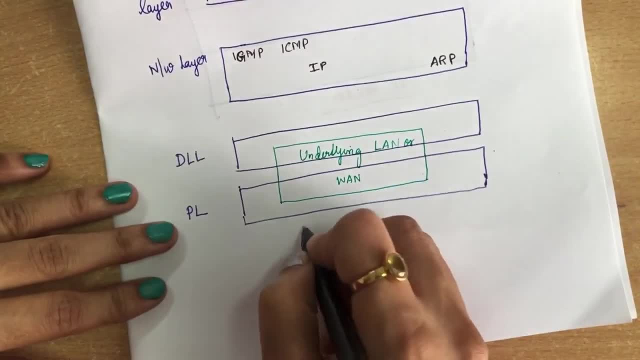 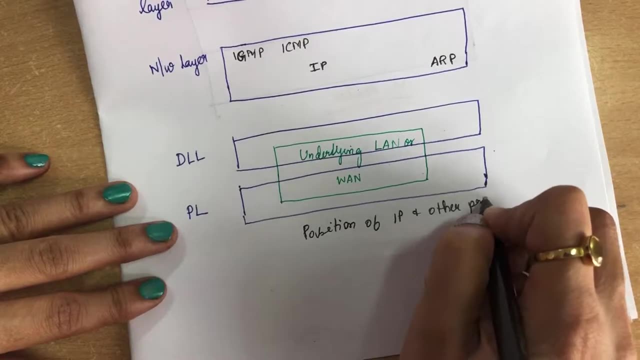 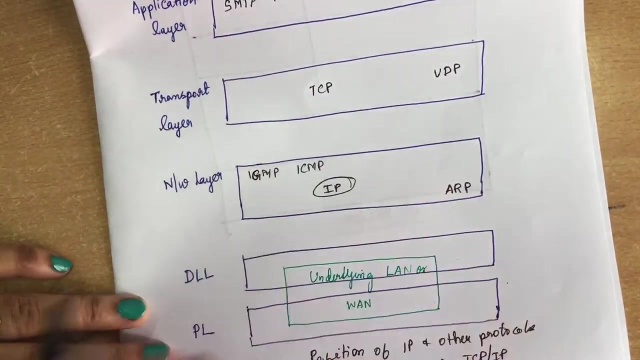 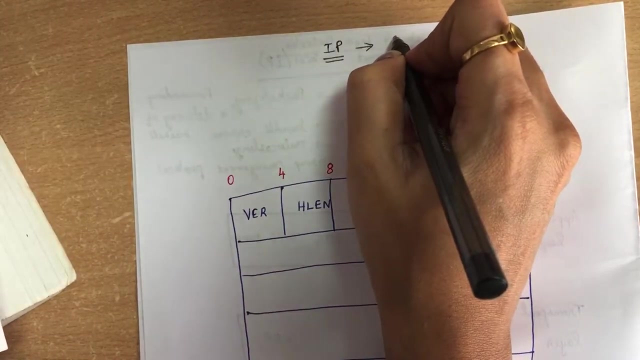 for the position of the. this is a diagram for the position of ip and other protocols in calls in tcp ip layer. okay, now we are going to see only about internet protocol, next coming to this ip protocol. so, coming to ip protocol, it is a unreliable. it's unreliable datagram service. it is. 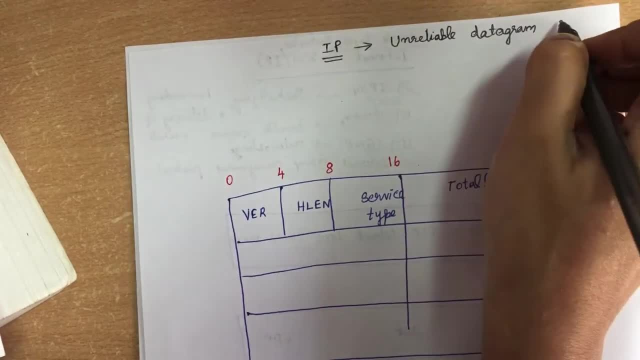 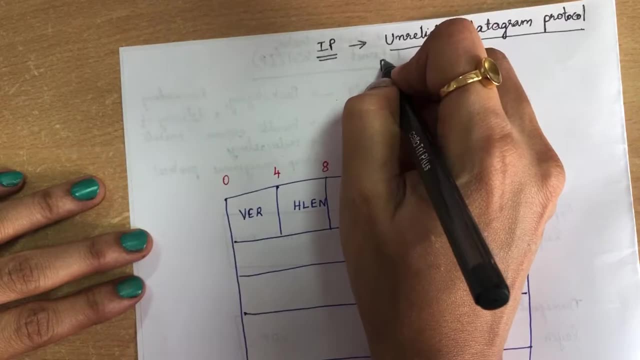 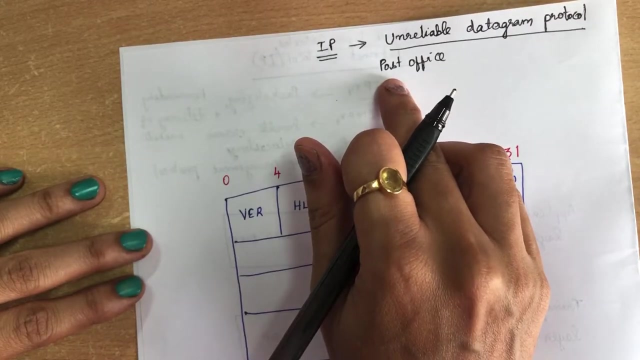 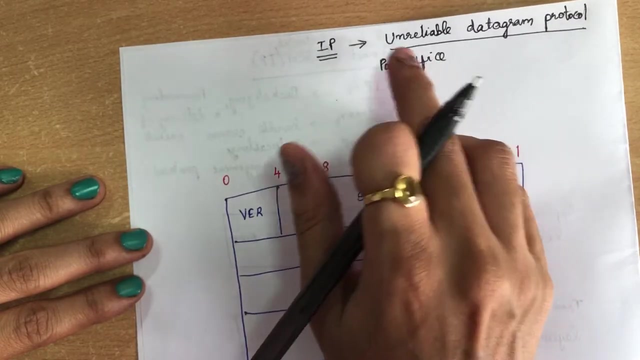 an unreliable datagram protocol. what do you mean by unreliable datagram protocol? so unreliable means it is similar to a post office delivery. so when you are sending your letter through post, okay, what happens is the sender doesn't know whether the letter has been received properly to the, it has been sent properly to the destination or not. similarly, this internet. 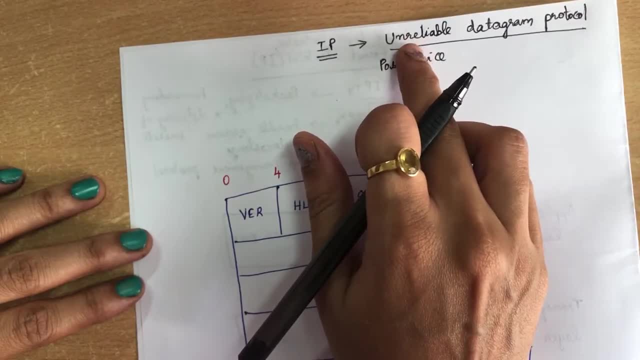 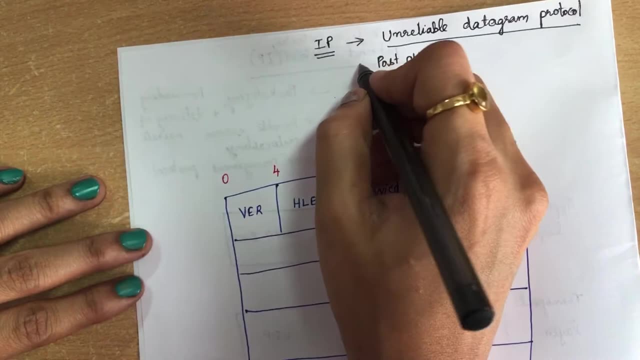 protocol also. it is unreliable, so if it doesn't know whether the package has been reached properly to the destination, so it is called unreliable. it is a datagram protocol. so if you want to make this to be a best effort each, if you want to make the delivery to be in best effort, 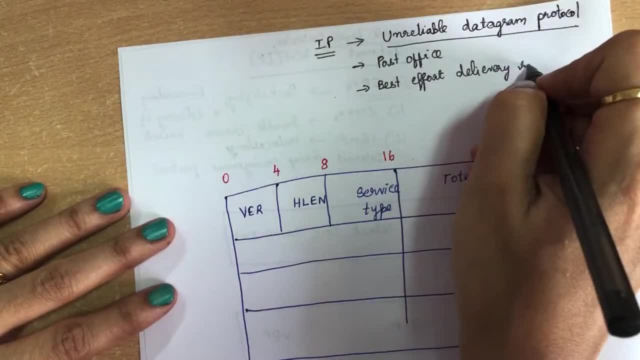 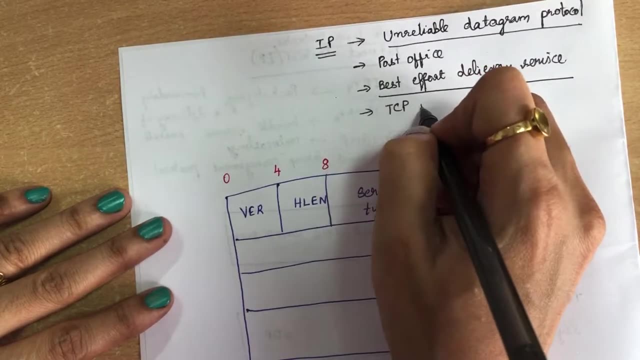 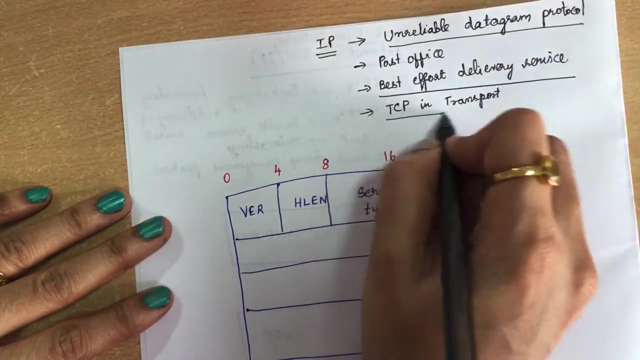 delivery service. so what you have to do is that usually this: you should pair it with tcp protocol in tcp protocol in transport layer. okay, in transport layer you have a tcp protocol. so if this ip protocol paired with tcp protocol, then you will get the best effort delivery service. 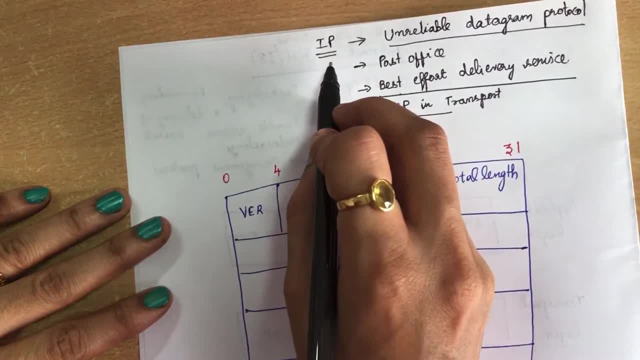 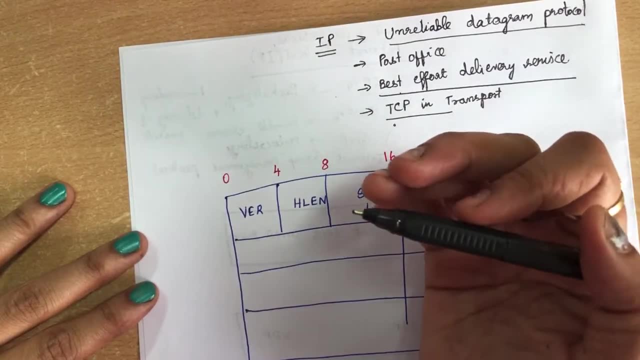 what do you mean by best effort delivery services? usually ip packets get lost, or it will be out of order, or the packets may be corrupted, or it can. there will be some congestion occur, so the packets will not be reached to the destination properly. in that case, if you are going to send a letter to the destination. if you are going to, if you are going to couple this ip protocol with tcp protocol, then your packets will be delivered properly to the destination, without any delay, or without any congestion, or without any corruption. okay, this is what is. it will provide you a best effort delivery. 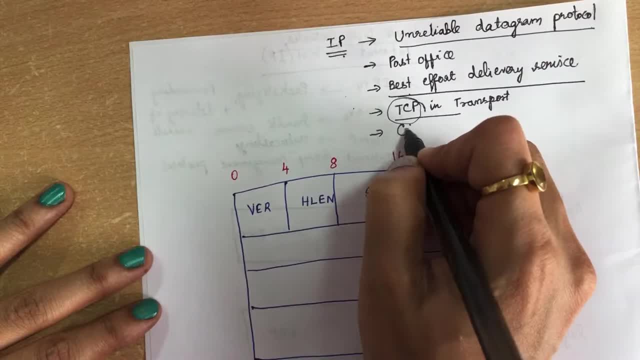 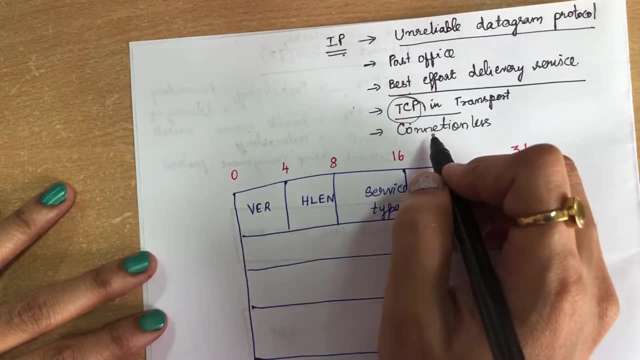 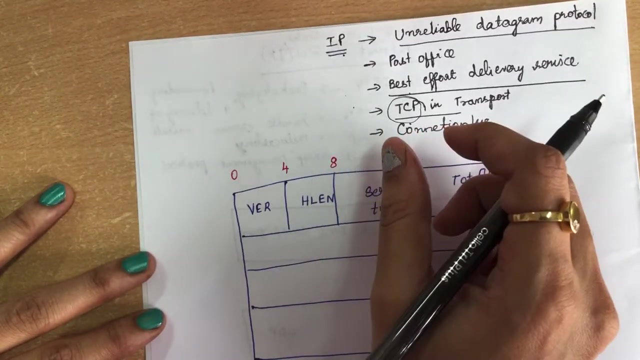 service and we can also say ip protocol to be it is a connectionless protocol also. so here what happens is like we are not going to establish the connection and we are going to send the data, so it is a connectionless service. all the packets, it will be all the datagrams here or independent, so there will not be a connection. 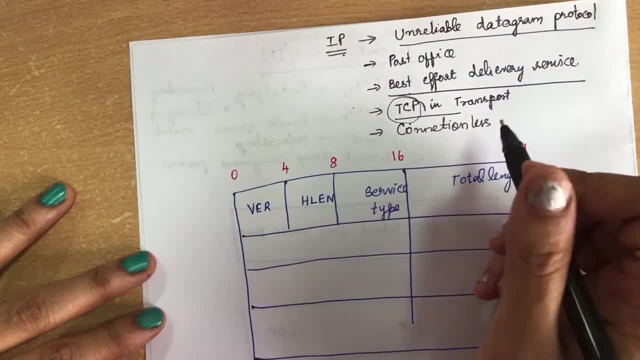 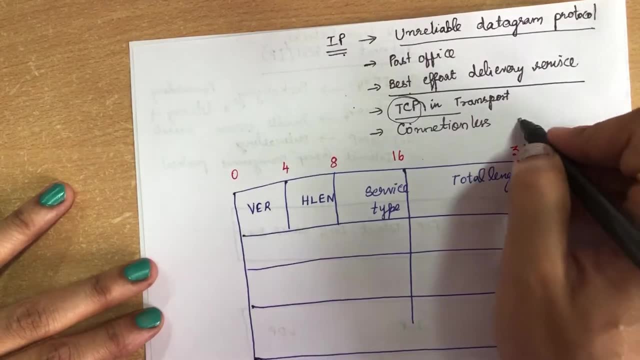 connection will not be there between all the datagrams. so what happens is they will take all the datagrams. they can use any path to reach a destination. so if they are going in different paths- different paths- and they will- they can. the destination, all the datagrams can be out of order. also so we can say: ip protocol is an unreliable datagram protocol. it is a connectionless protocol. if you want to give a best effort delivery service, then you can couple tcp protocol with ip. it will give you the best effort delivery service. okay, we will see what is. the main function of internet protocol is packetizing. so we will see the first. 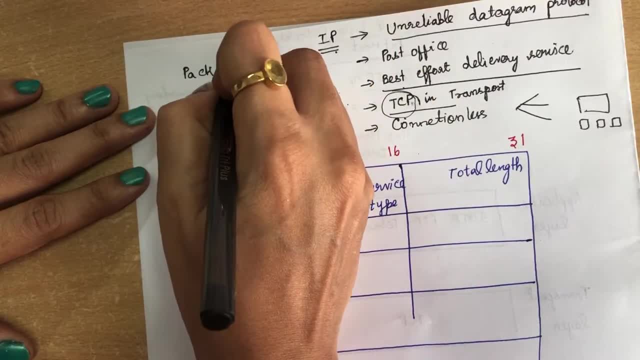 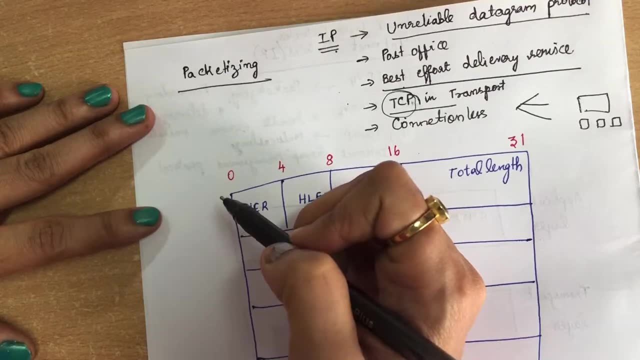 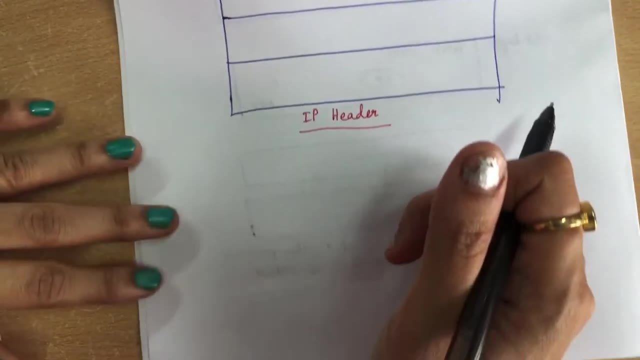 service that is provided by ip, that is packetizing. so the packets coming from the higher layer, higher layer- it will be passed to the network layer. so in this network layer the packet format only we are going to see it now. so here the packets are called as datagram. in network layer packets are: 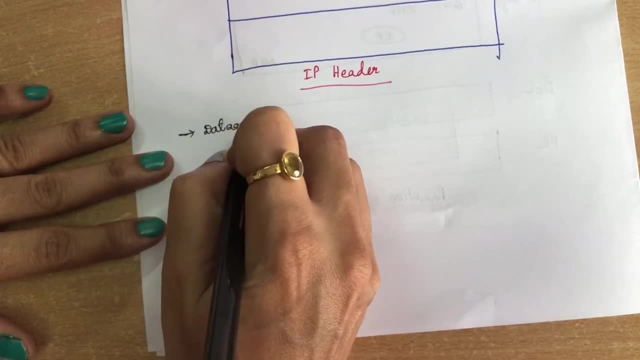 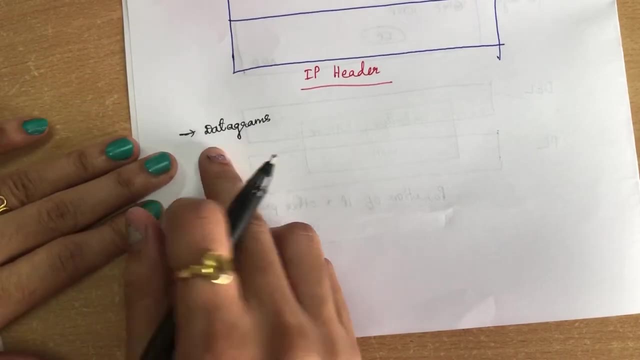 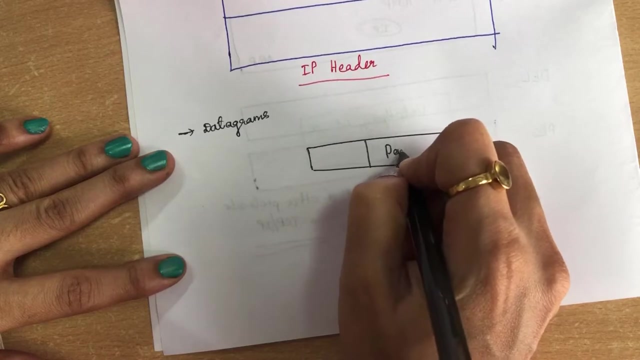 called as datagrams. so the packets are called as datagrams, but in but in case of your data link layer, it is called as frame, so it is datagrams. so usually if you consider an ip datagram, so it will contain a data that is called as payload. here it is called as payload and you had and header, so 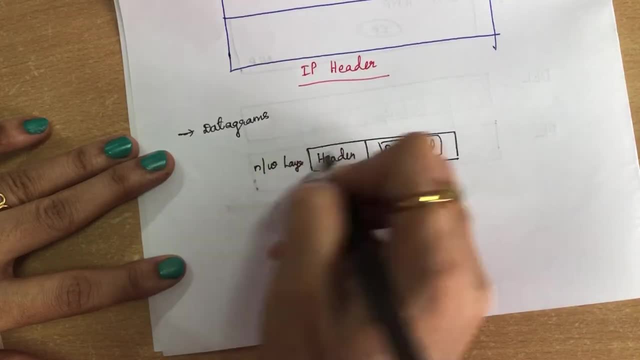 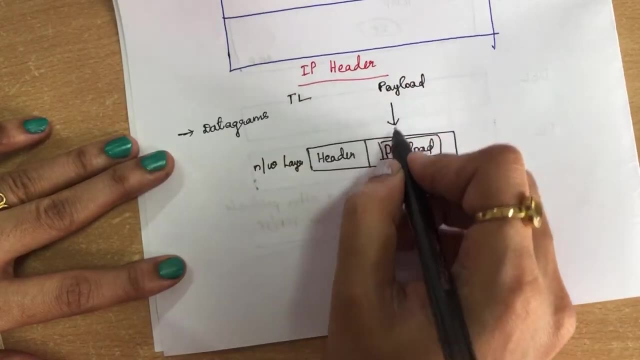 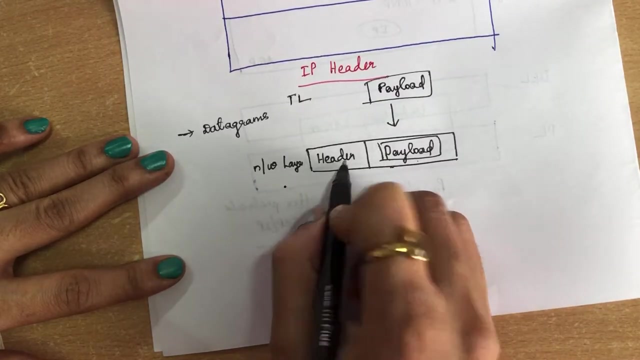 the network layer. what it does is network layer. it will get the data day, that is, a payload or data, from the transport layer. okay, it will get the payload or data from the transport layer, the network layer. it will add its own header to this data, so the header will be of size 20 bytes to 60 bytes. 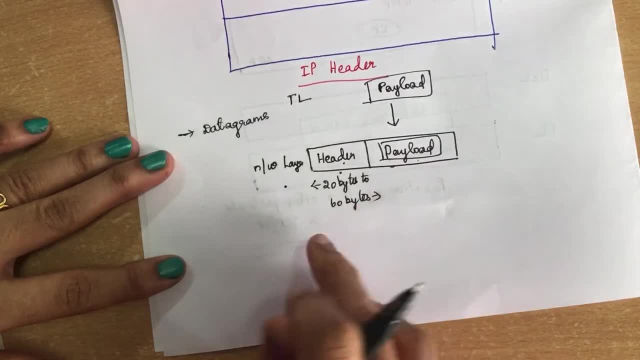 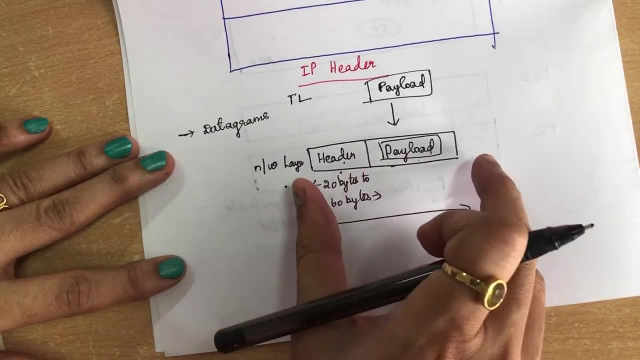 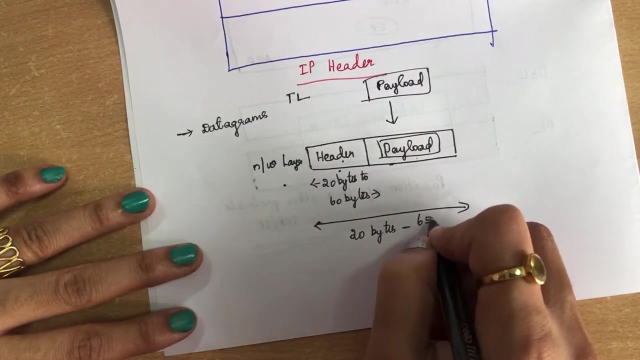 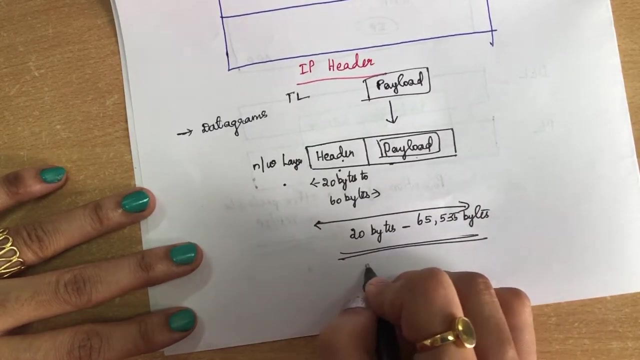 so the length of the header will be 20 bytes to 60 bytes. and what is the length of the data? entire datagram, that is, this one entire datagram. it will be of the size 20 bytes, starting from 20 bytes to 65,535 bytes. so this is your the length of entire datagram. this is the IP datagram. 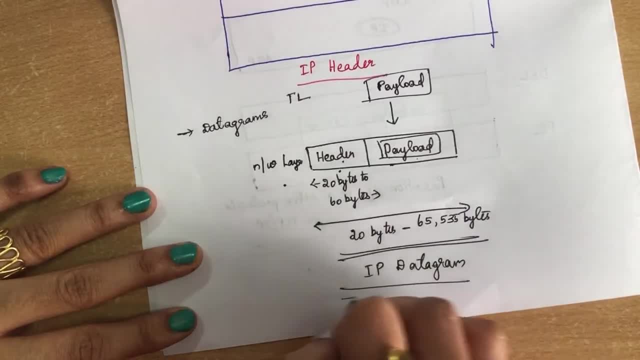 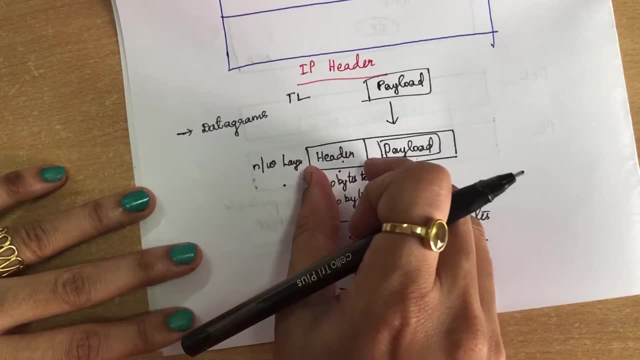 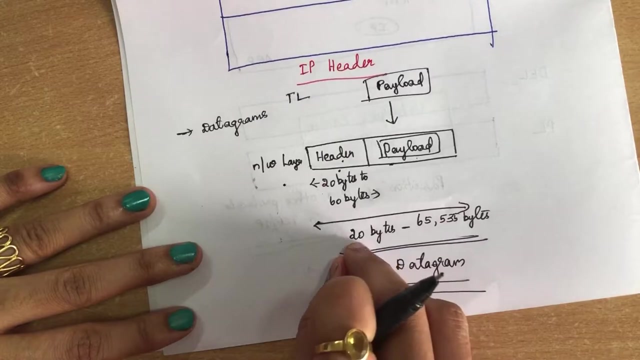 so coming to IP datagram, so the data it will add. the header data link layer will add its own header and trailer, but here network layer will add only the header. header will be of length 20 bytes to 60 bytes, so the entire length of the network layer will be 20 bytes to 65,535 bytes. 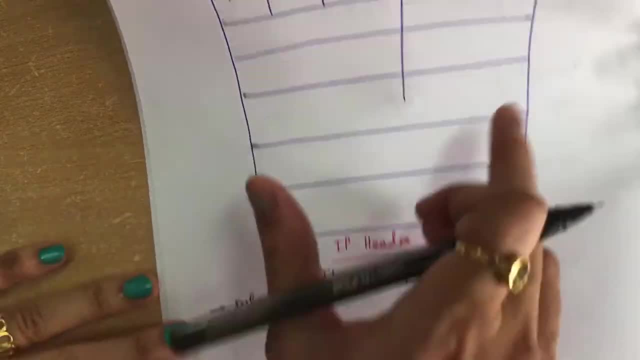 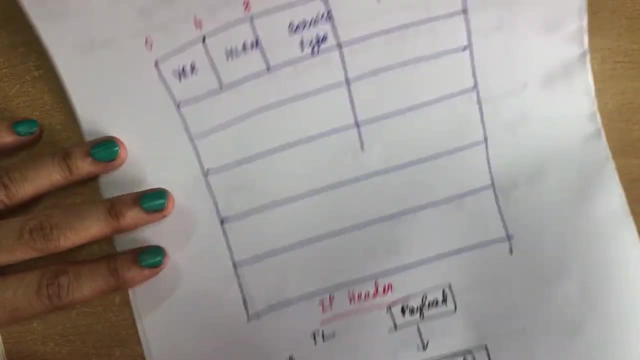 okay, so now we will see the header format now. so now we will see this header format. so this header, this header I have told you like it is of 20 bytes to 60 bytes. so now we will see what is the, what, all the information you have to keep it in the header. so the header, first, it will have the. 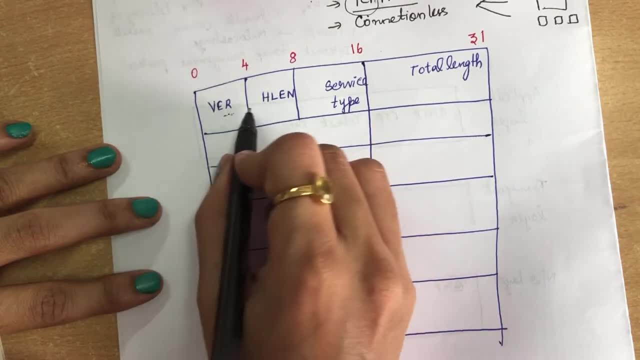 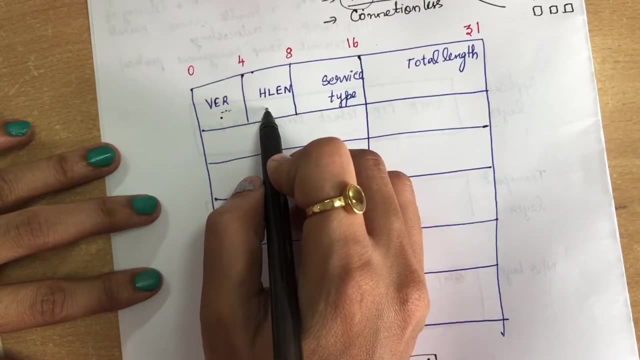 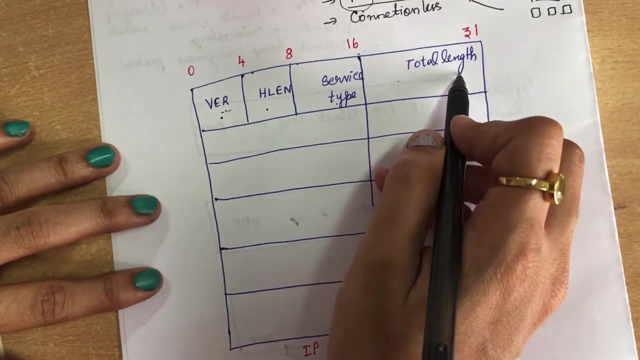 version number, header length. I will explain to you later. so first we will see what all the fields you have in your header, so version number and next 4 bits will be occupied by header length. next 18 bits is going to be occupied by service type. next 16 bits is occupied by total length and next, 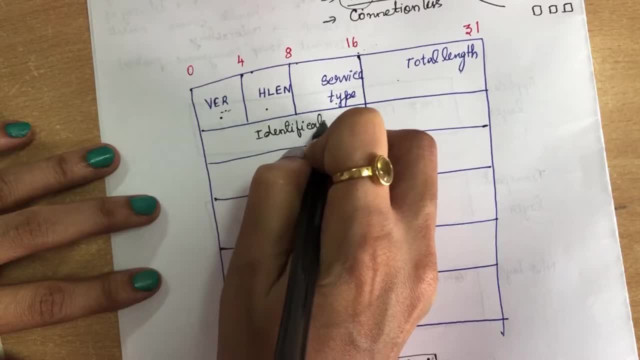 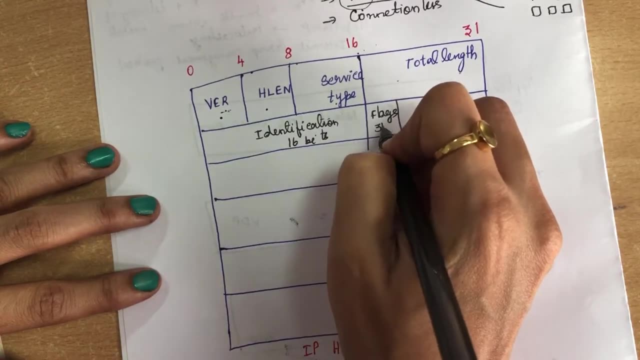 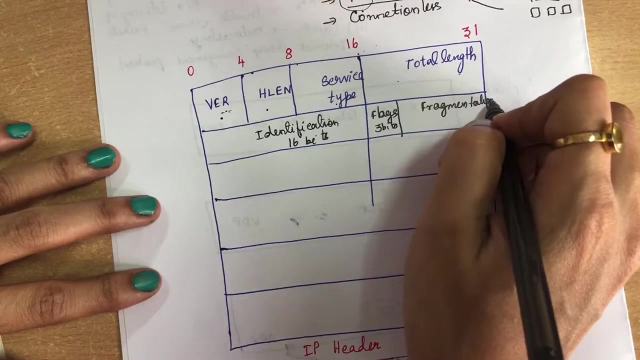 you have your identification number. okay, this is identification number, which is of 16 bits, okay. next you have your flags, that is of 3 bits, and next you have your fragmentation, since this network layer also helps in fragmentation, so it is fragmentation. offset is placed over here. it is of 13 bits, so totally 16 bits is there. 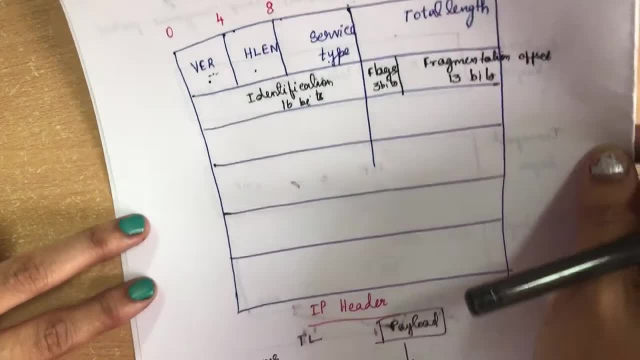 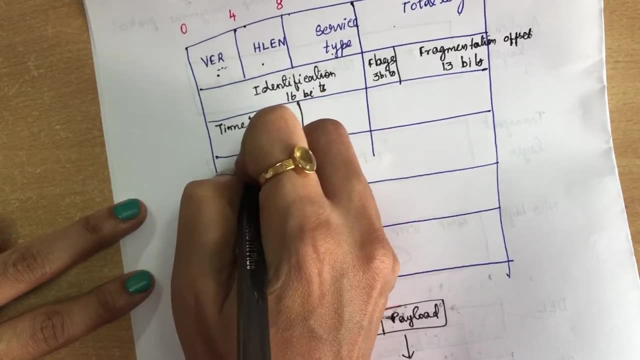 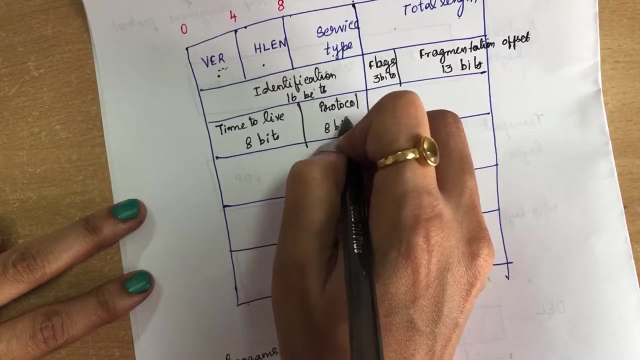 occupied by flats and remaining 13 bits is occupied by fragmentation offset, and you have here time to live, okay, time to live, value, which is of 8 bits. and next you have a protocol. which protocol you are going to use it for transmission? that is also, which is of 8 bits. next you have 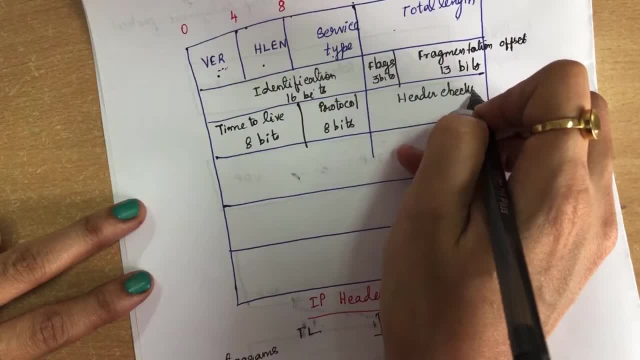 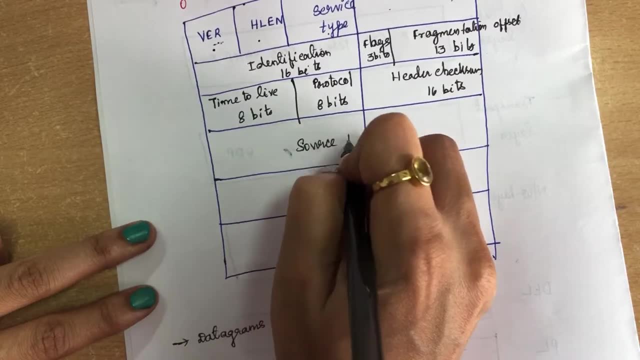 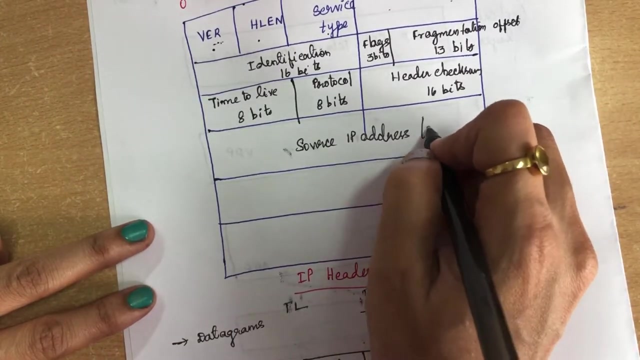 your header checksum. okay, checksum which is of 16 bits. okay, these are the fields. next field is source ip address. source ip address. you need a source and ip address to identify where that particular packet has been sent from, so which is of 32 bits. next you have your destination ip address. 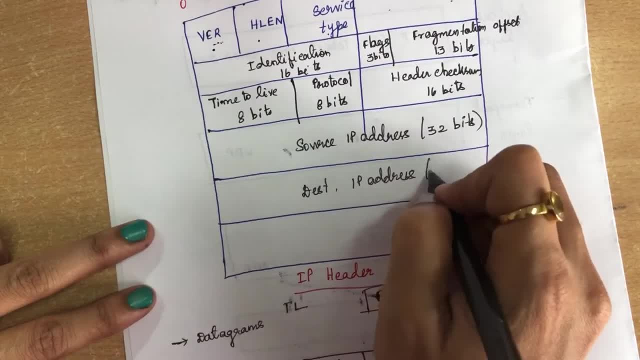 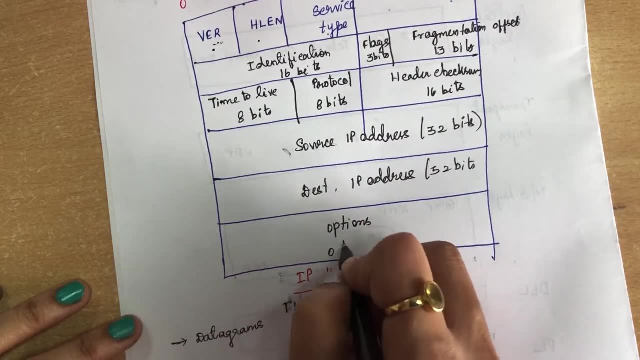 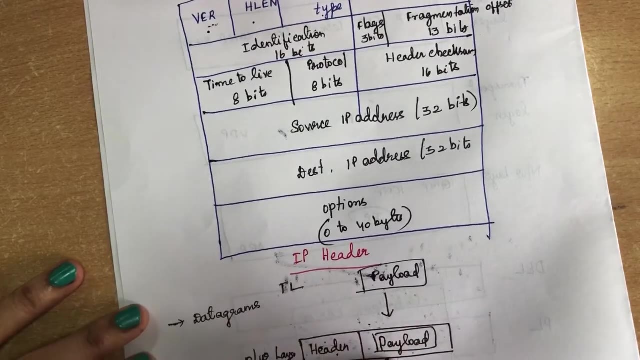 that is also 32 bits. last is options: okay, so this will be of 0 to 40 bytes. okay, this is what you have. this is these are the information. you have to add it with along with your data. so first is version: header length. service type: total length. 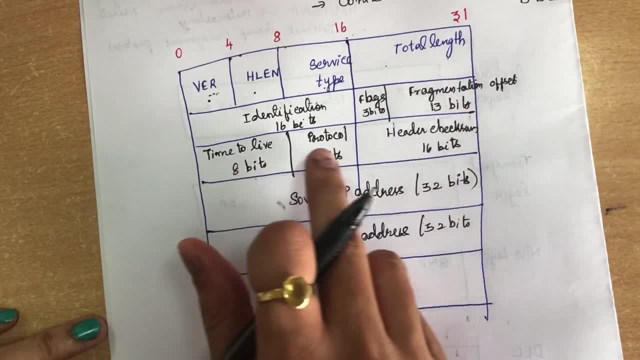 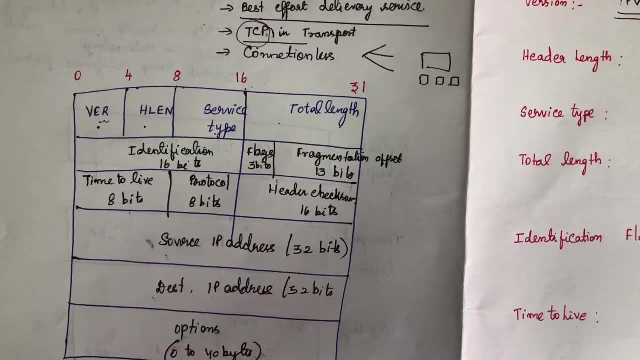 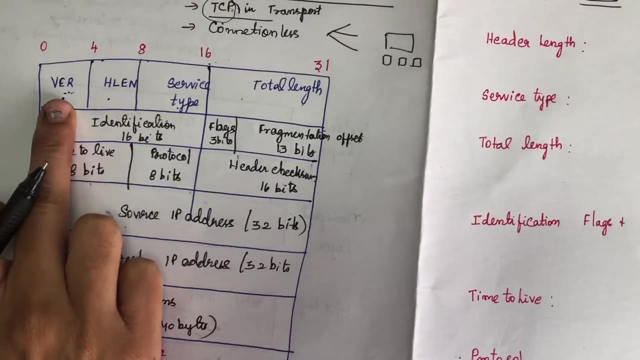 identification number, flats, fragmentation, offset, time to live, protocol header checksum, source, ip address, destination, ip address and options. okay, we will see one by one now. now i will explain about the fields of ip header. first, coming to the version. okay, this version defines the ip version 4 protocol. so the version which you are using for ip protocol is version 4, that number. 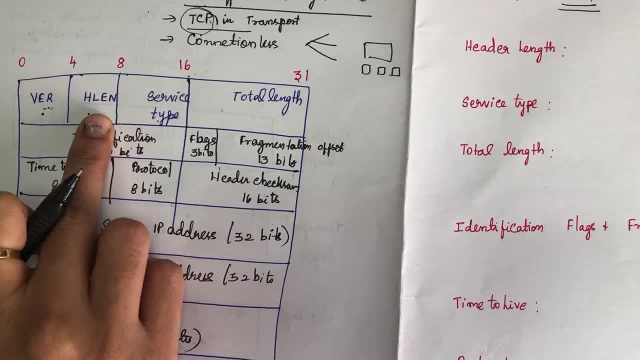 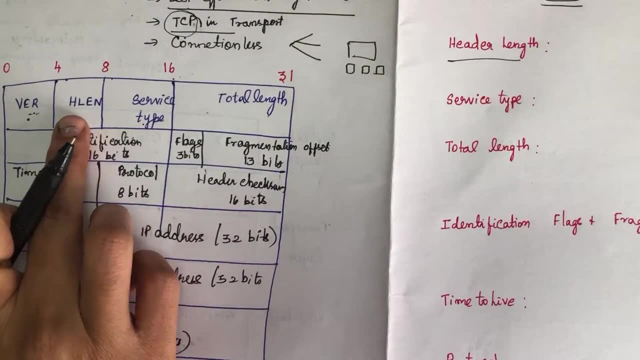 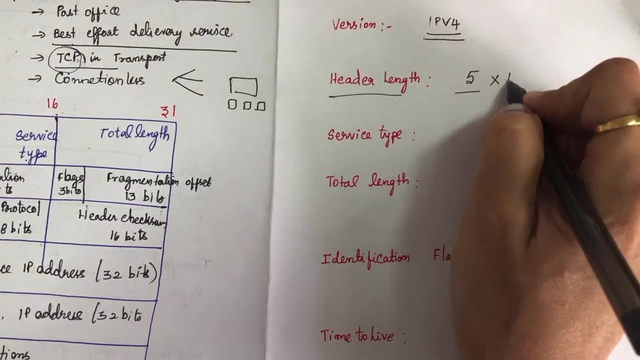 here with 4 bits. next comes your header length. header length specifies the length of the header. usually this is this has to be. this length should be fit into this 4 bits. so usually, suppose, if the header length is 5, what the receiver has to do is he has to multiply this value by 4, so that value 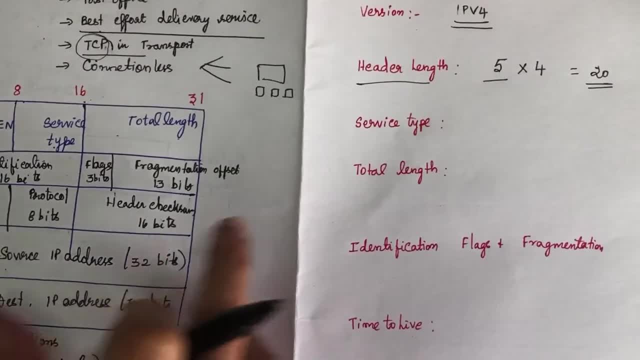 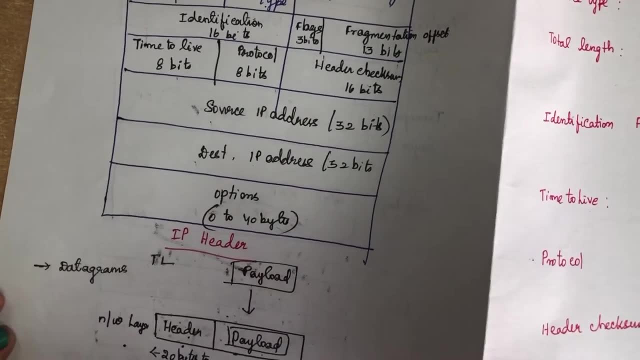 will give you the value called 20 bytes. so the length of the header is 20 bytes. so here, actual length of the header may be from 20 bytes to 60 bytes. 20 bytes to 60 bytes. as we have already seen the length of the header, it will be from: 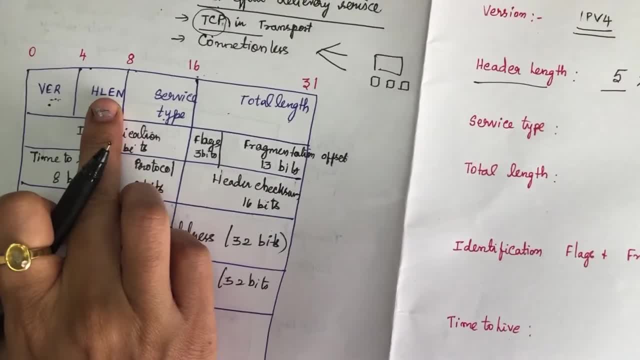 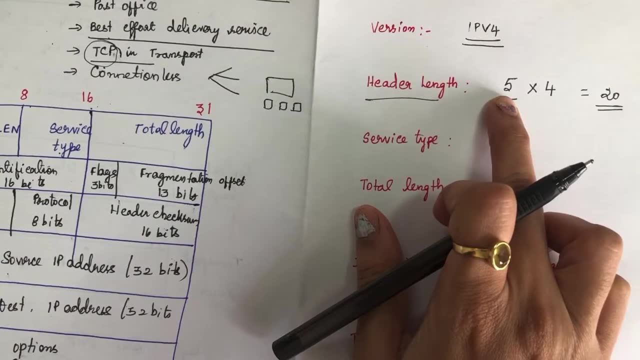 20 to 60 bytes. so here, if the value of the header length is 5 over here, given here, since it has to fit within the 4 bits they have given this number. suppose if, if the the value specified here is 5, the receiver has to multiply this number by 4 so that so that actual length 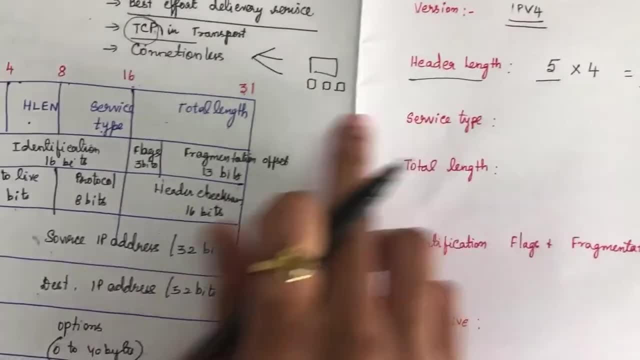 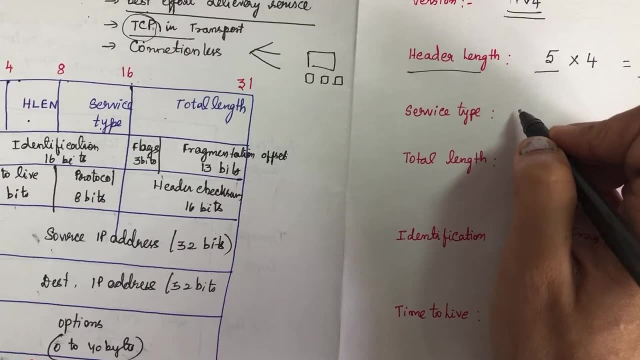 of the header can be found. okay, next give you. next is service type. service type will tell you the type of the datagram. what type of service is service type? service type will be this particular ip is going to provide for you. that is the service type. next is total length. 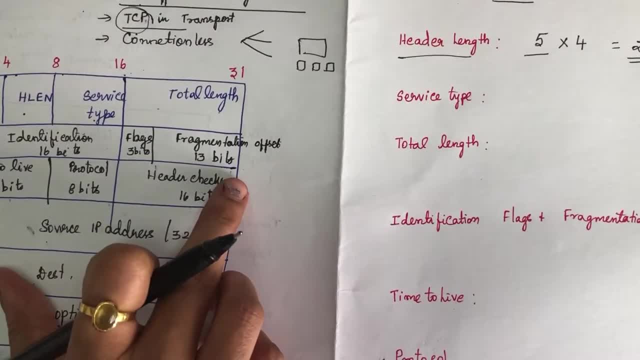 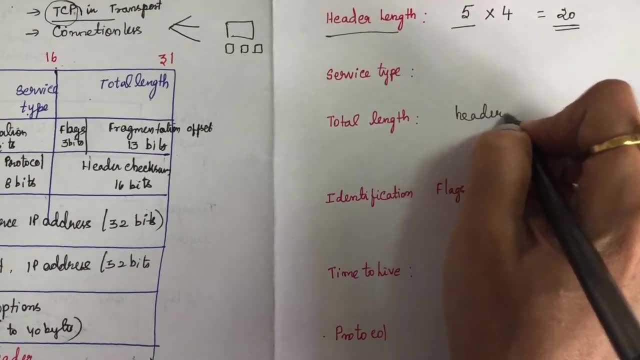 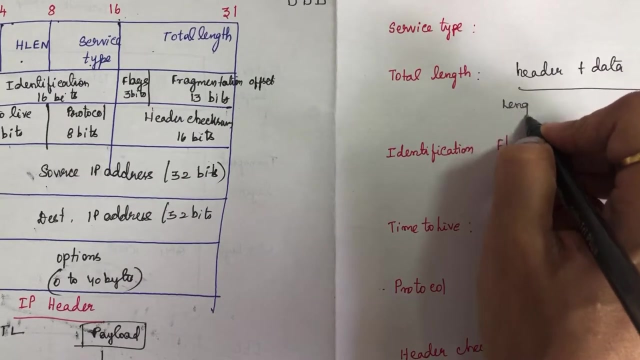 coming to the total length of the. this total length of the data, that is. here. the total length defines both the header and also plus data. here the total length is nothing but the header plus data. okay, so if you want to calculate the length of the data, so how will you calculate the length? 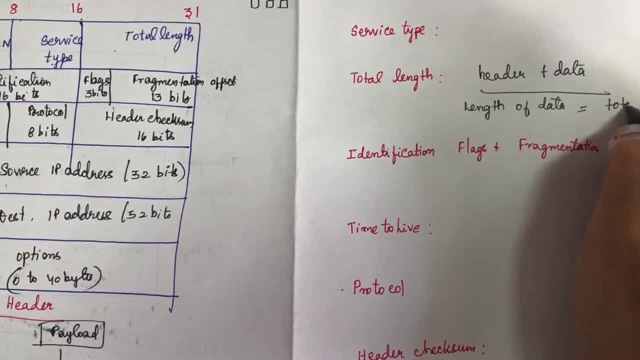 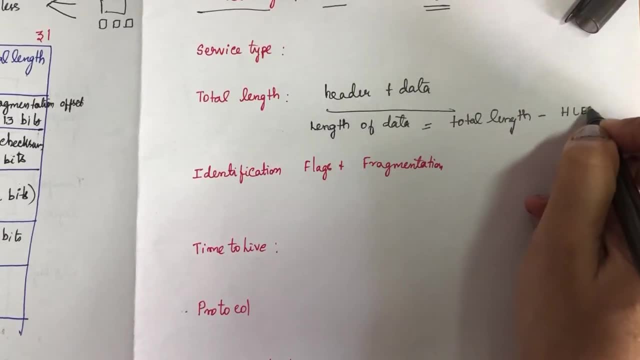 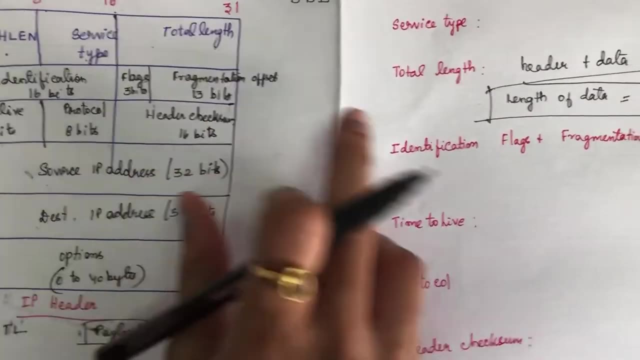 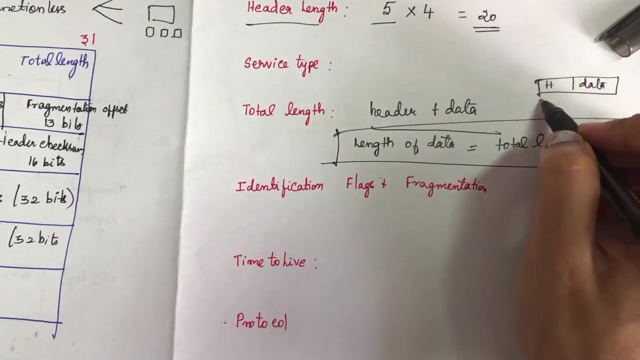 of the data alone, that will be nothing but this total length, this total length minus this h length, h length is the header length into 4. so when you calculate this value, you can find out the value for total length of the data alone. so as, actually, we know that you have a header and you have a data, so here the total length, here this: 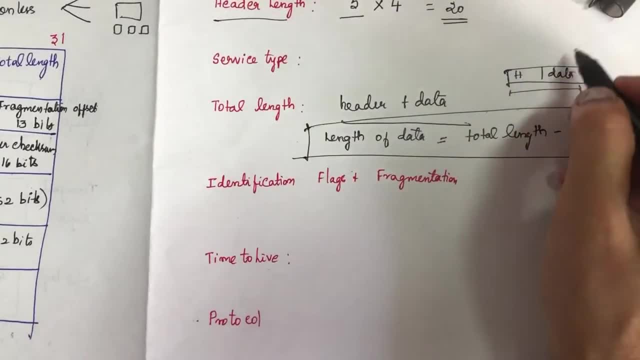 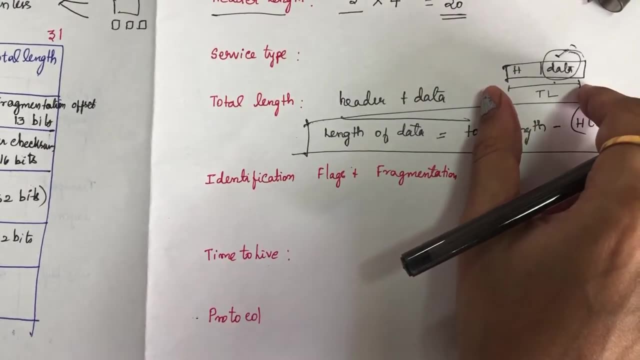 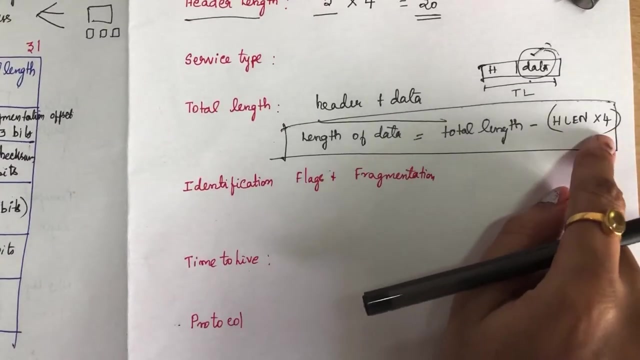 value specifies the length of both the header and data, suppose if you want to find out this length of the data alone. so what you have to do is you have to subtract the value's total length from this, the this header length. so header length. you have to multiply by 4 that header length into 4 that. 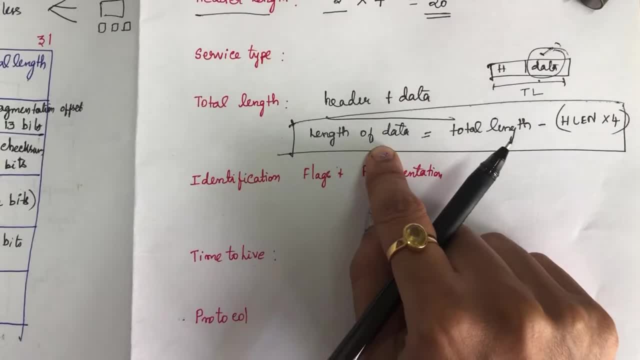 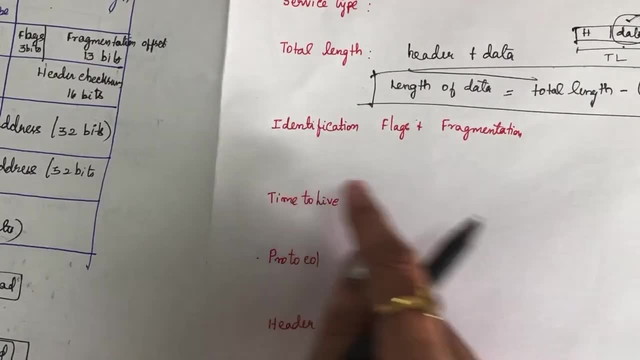 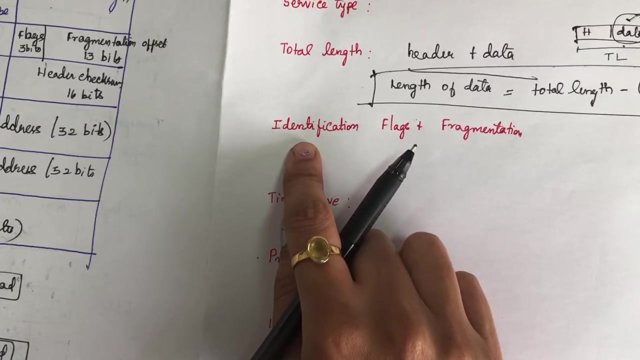 subtracted from the total length will give you the length of the data alone. okay, next is identification flags and fragmentation. this we will. i will explain all these three things later after this topic. okay, so these are used for fragmentation. identification is used to forgive the identification number for each. 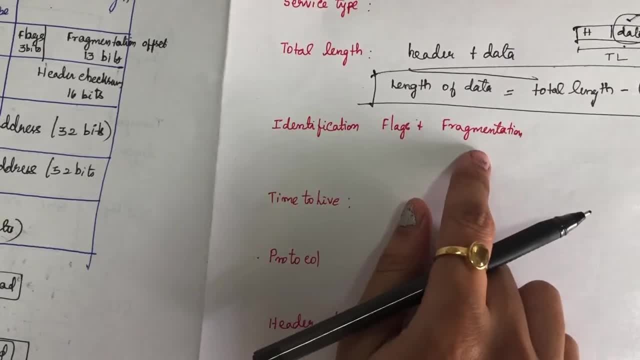 datagram packet that is the identification number, to prove the fact of what kind of етров this be looked like this. i will j advisory here later. okay, how it is &id is is that the maqr暱 p? Uhh: identification and flags and fragmentation. i'll explain to you later. next is time to live time. 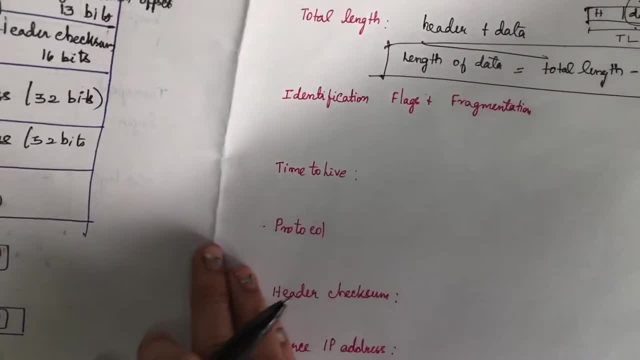 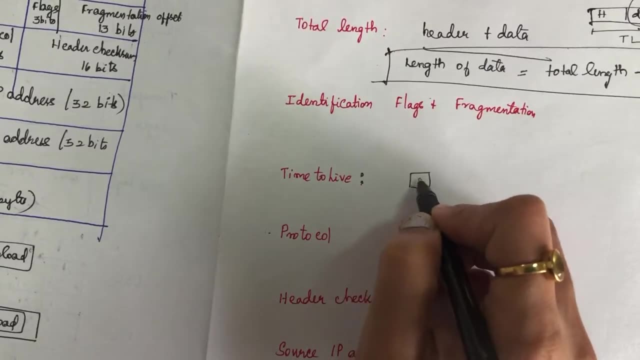 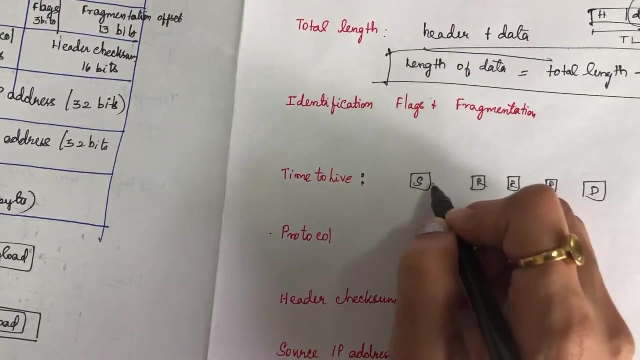 to live value this time. to live value, it is nothing but a value, which is which will be created whenever a datagram is created, usually suppose, for example, you have a source and here you have a destination. in between, you have so many routers- okay, router one, router two, router three, so what? 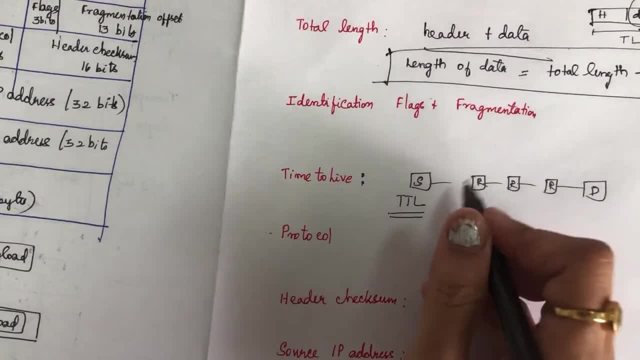 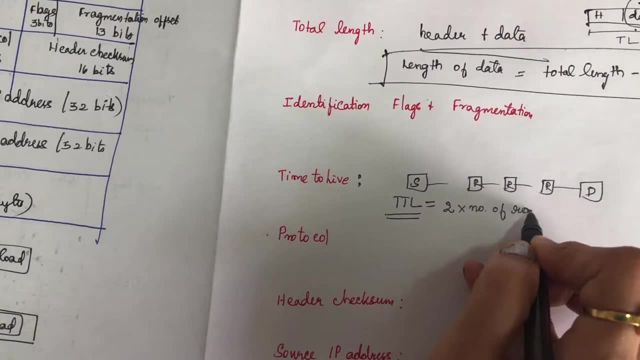 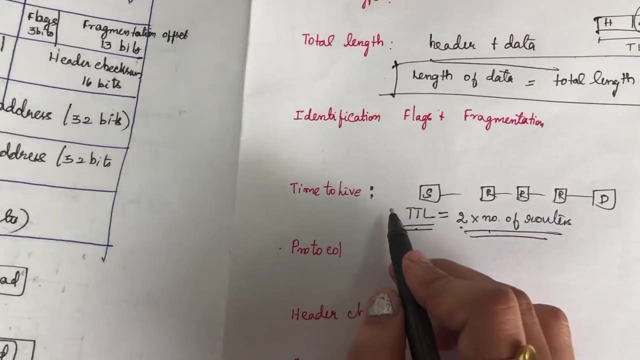 happens is this time to live period. it will be set by the sender this value. it will be, it will. this value. it is nothing but twice the number of routers. okay, twice the number of routers: okay. this value will be set, with the value of two, into number of routers in your network, so that 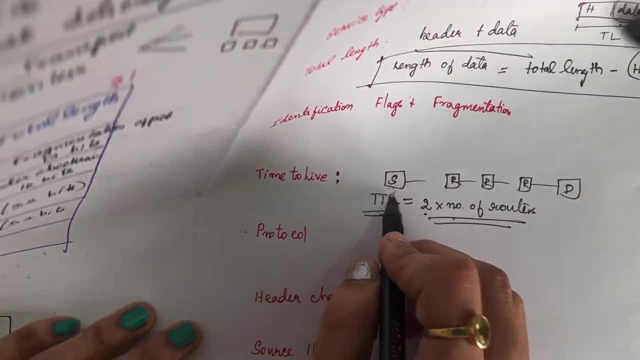 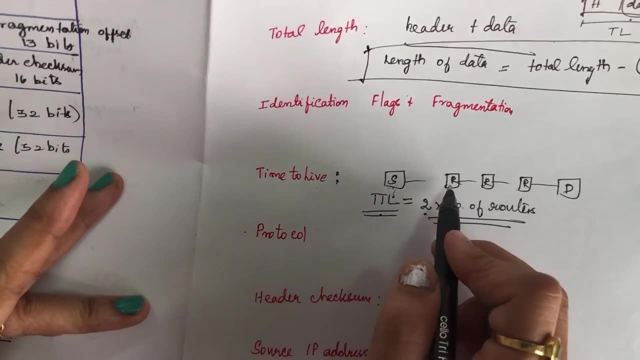 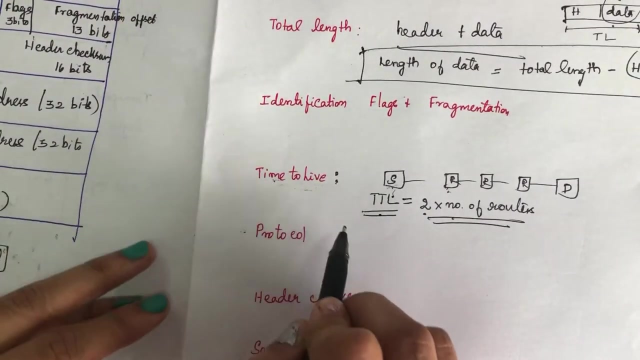 value will be set over here. every time this packet or datagram reaches your next hop, this ttl value will be decremented. likewise, it goes on decrementing. once this ttl value is become zero, then the packet or datagram will be discarded. okay, this is the function for time to live value. 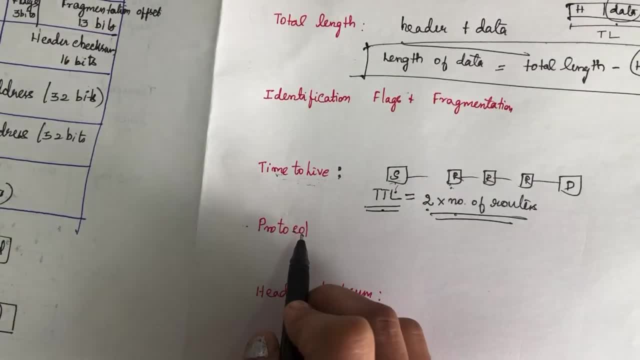 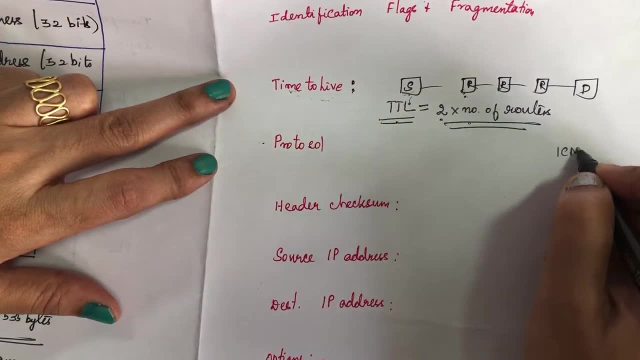 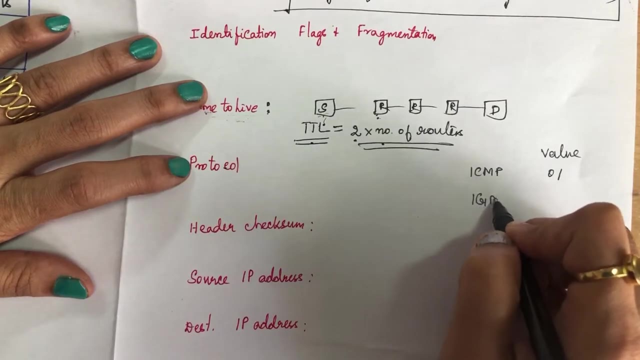 okay. next is protocol. coming to the protocol. so we need to know what type of protocol we are going to use it for sending the packet. so for this we have given some values for this. if you are going to use icmp protocol, the value for this is 0, 1, okay. and if you are going to use igmp protocol, 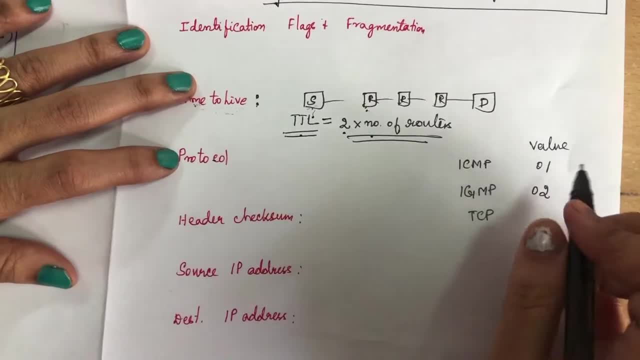 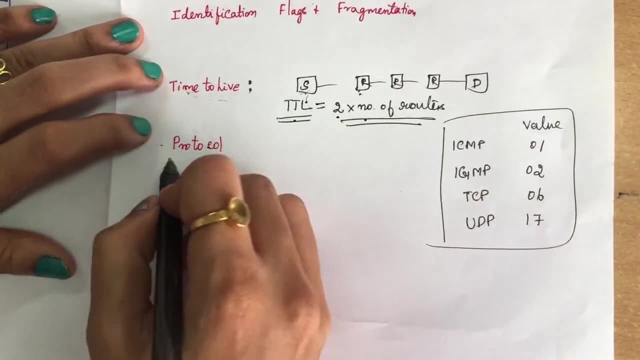 it is 0- 2, and if you are going to make use of pcb protocol while you are sending the packet, it is 0- 6 and udp protocol it is 0- 17. so these are the values you have to mention in protocol. so this protocol you have, several values are given so you can make use of all these values. 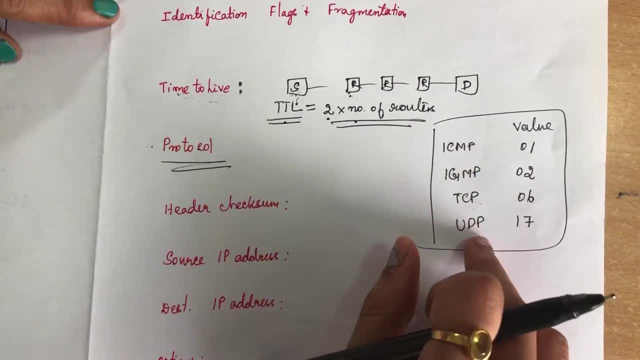 to specify in this protocol, whichever protocol which you are going to use it along with ip protocol. you can mention it. whether ic internet control message protocol means 0, 1, internet group management protocol, it is 0- 2. if you are going to couple with the transport control protocol, it is. 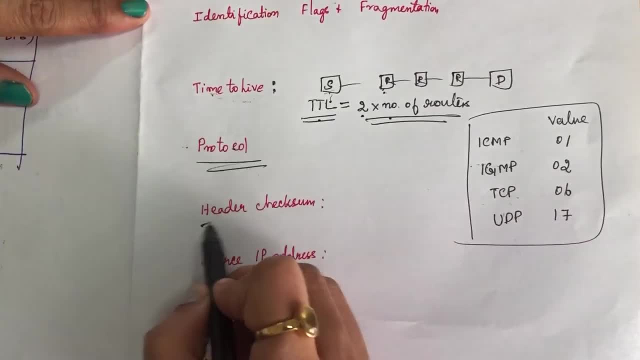 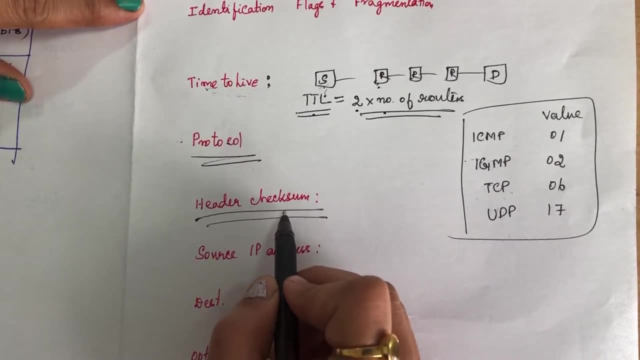 0, 6 and user datagram protocol: it is 17. okay, next is header checksum. so, since we all know that the packet can be corrupted or it can be corrupted, it can be corrupted, so we need to know that the packet can be lost. so, for that purpose, so to do the error correction and error correction, 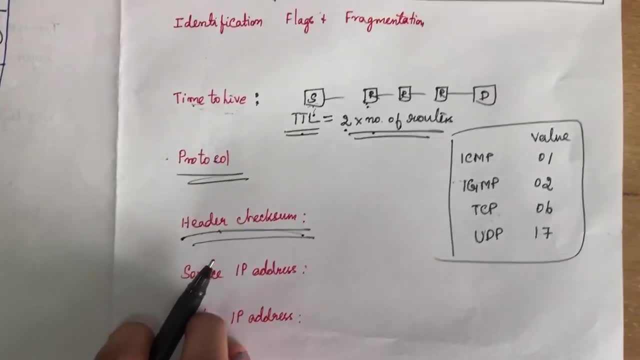 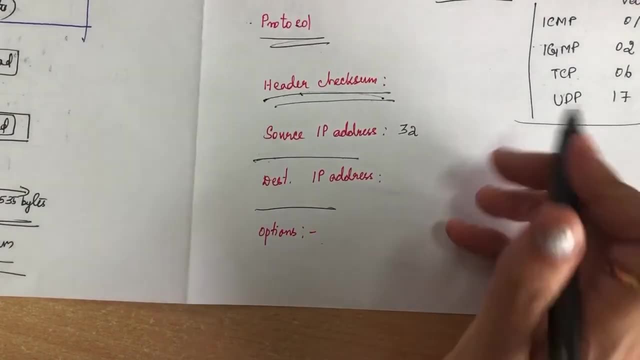 and reduction. we are going to have enter checksum that will also explain to you after this. okay, and next comes your source ip address and destination ip address. this is of 32 bits, as we all know. ip address will be, will be specified with help of 32 bits, so we have to give the exact 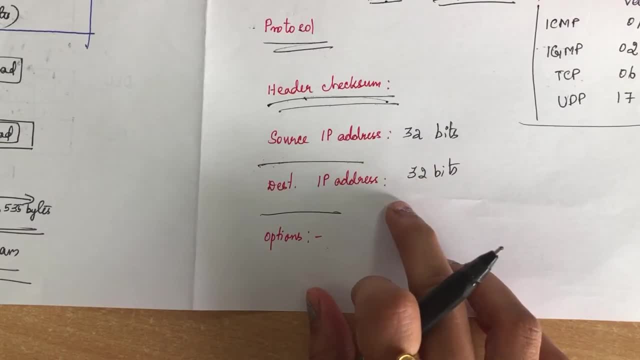 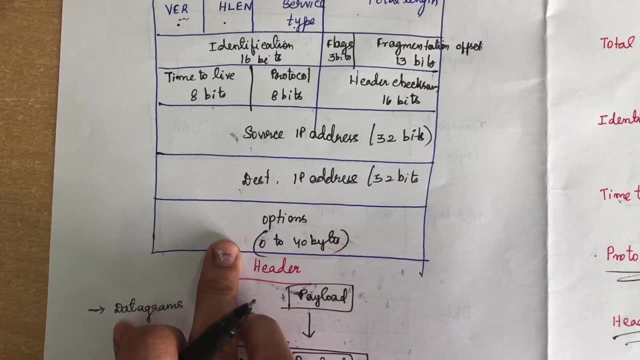 source address from which you are going to send the data and to which destination you have to you are going to send. so both this thing, it will be mentioned over here. so the options will tell you whether it may be any, any error correction. all these options, it will be specified over here. 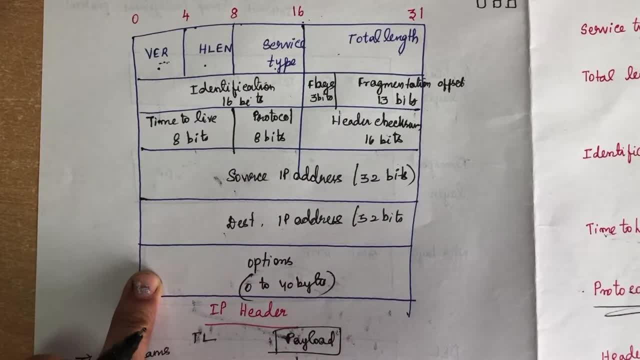 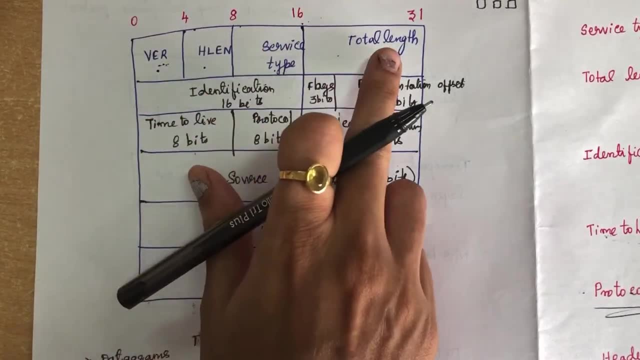 this is what you have, the fields in your ip header. okay, so, along with the data, you have to send this ip header which contains all this information- version number, header length, service type, total length- and you have an identification number, flags, fragmentation, offset, time to live period and then 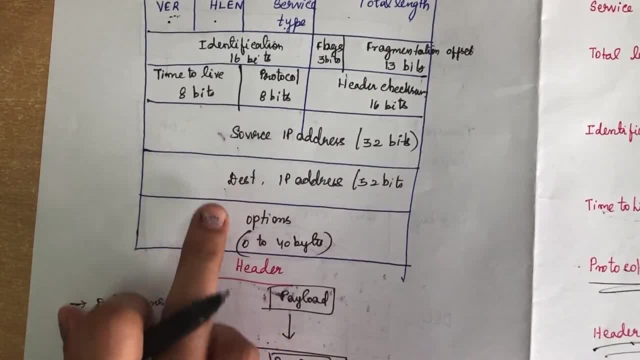 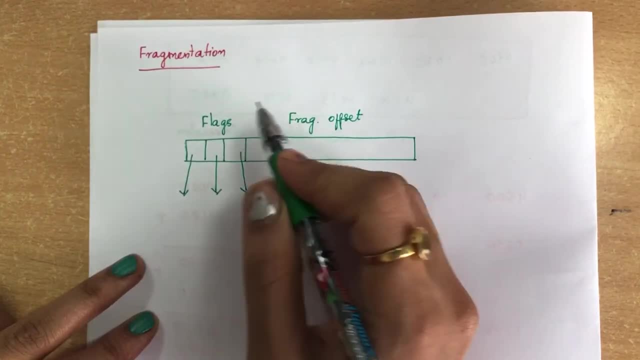 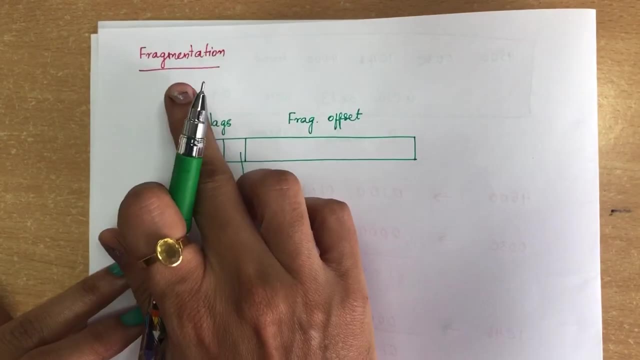 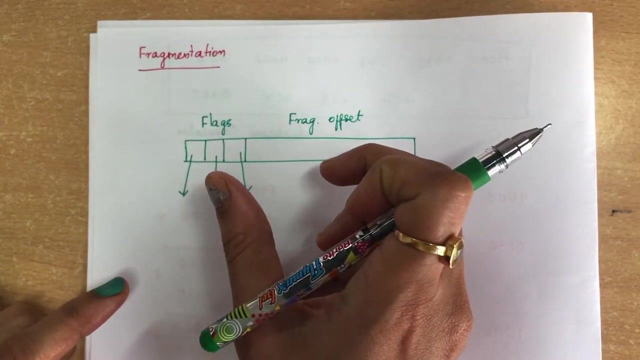 protocol you have to mention the header, checksum, source, ip address, destination ip address and options service provided by ip protocol is fragmentation. so what is fragmentation actually? whenever the data, if it exceeds the maximum, the length, so we need to do this fragmentation. so whenever fragmentation is done, the header is also added to each datagram. okay, that is what fragmentation is. 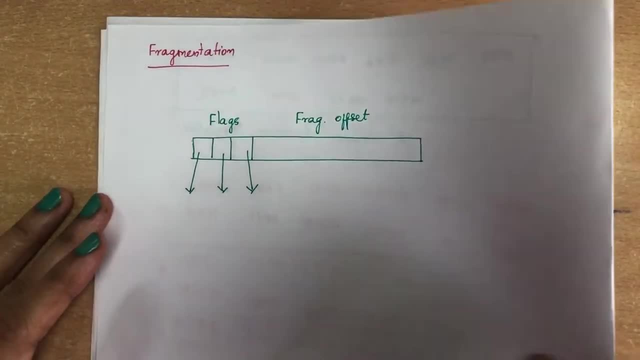 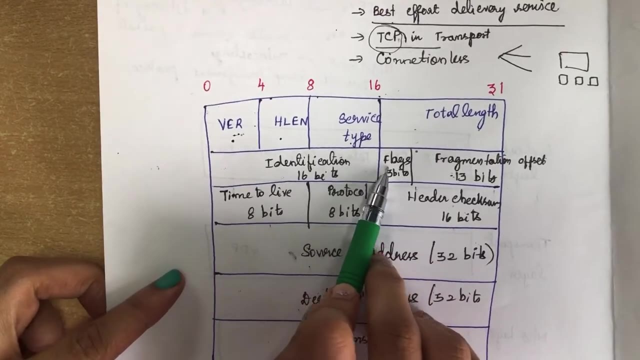 done so. first we will see what is. we already know that. that is like in the packet that is in the header we have a bit called flax. i told you like i will be explaining this- flax and also fragmentation also. that is what i am explaining now. this identification is a 16 bit identification. 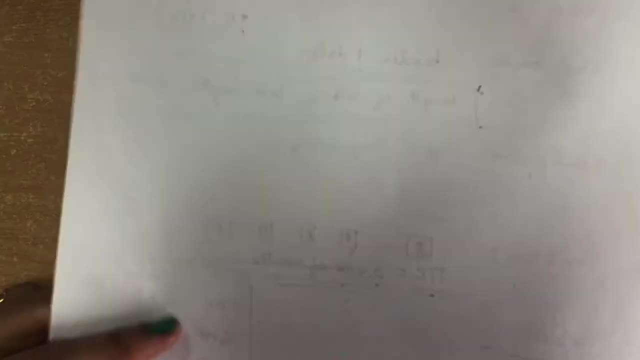 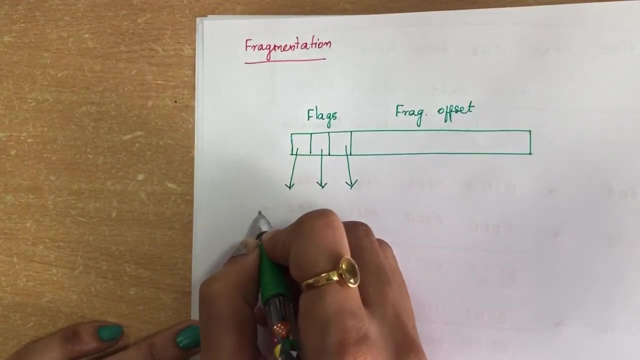 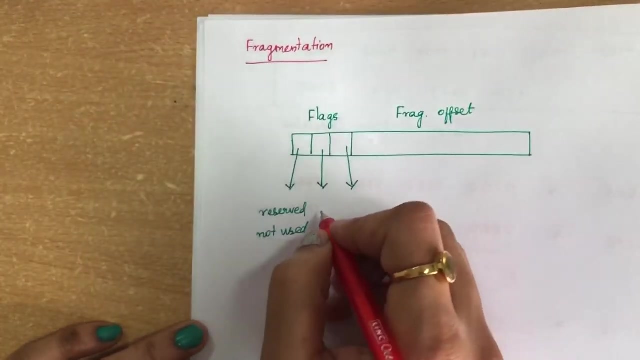 number which is given to each datagram. okay, so now we will see about this. the flax. so, coming to the flax, you have three bits. okay, the first bit is reserved, which is not used usually, so this is reserved and which is not used. the second bit, it is called as the d bit. okay, it is called d bit. 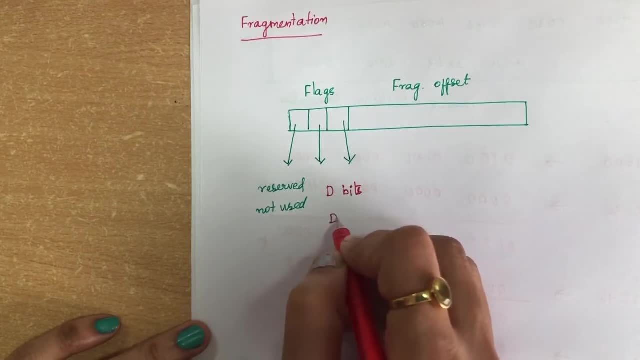 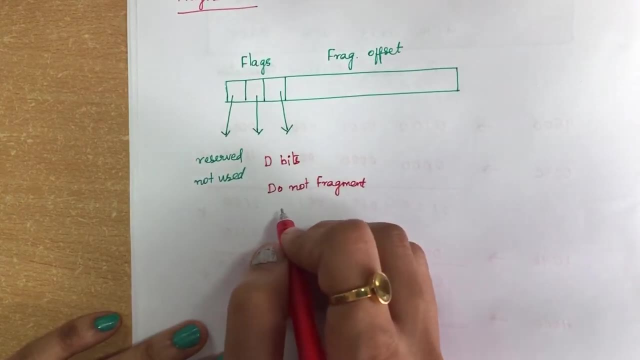 the second bit is called d bit. okay, the third bit is called d bit, so this is reserved and which is second bit is called as d bit and it is nothing but do not fragment. it means it is: do not fragment. okay, if you want the datagram not to be fragmented, you can give this value d bit to. 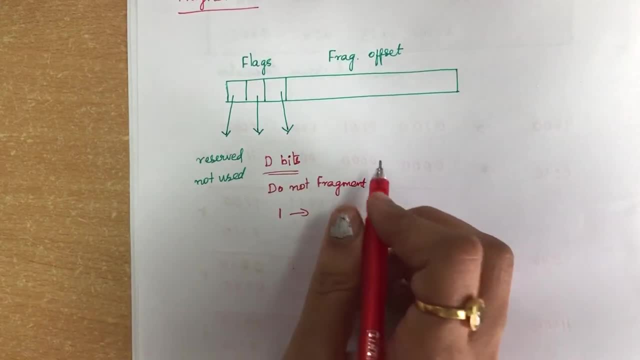 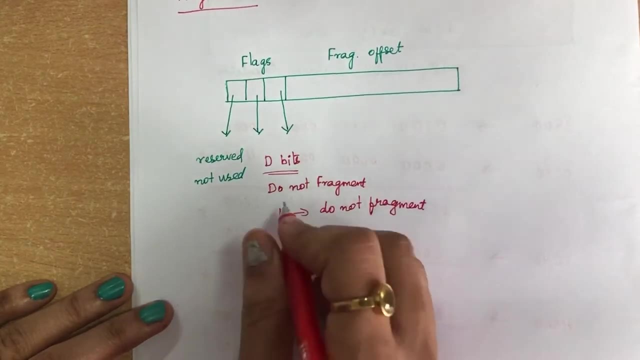 set this value 1, so when this d bit is set to 1, it means you cannot fragment the datagram. do not fragment, okay. fragmentation cannot be done. what do you mean by 0?? 0 means you can do. 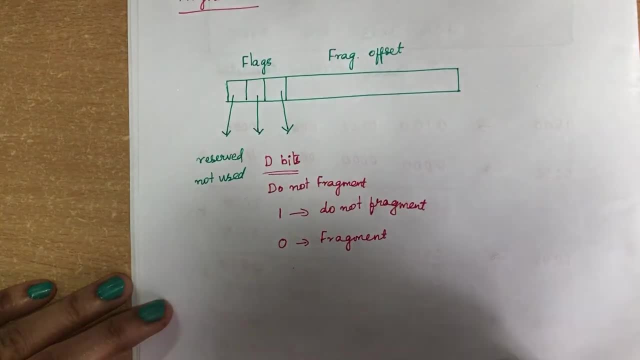 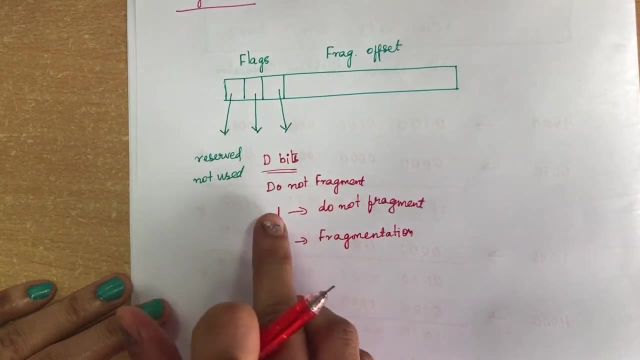 the fragmentation. that means you can divide the data into so many fragments. okay, this fragmentation can be done. so the d bit specifies it is called: do not fragment when it is 1, it is do not, you cannot fragment the datagram. if it is 0, you can fragment the datagram. 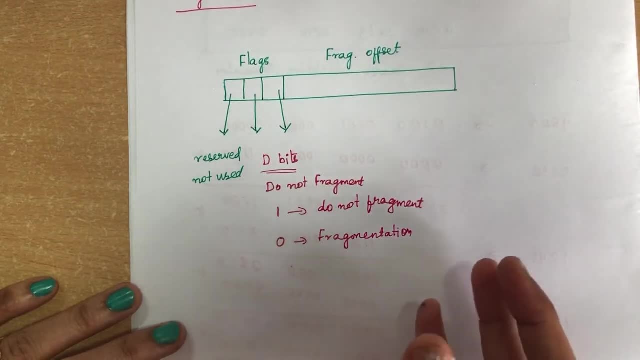 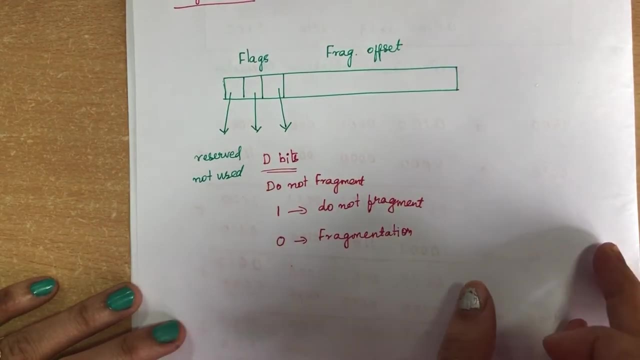 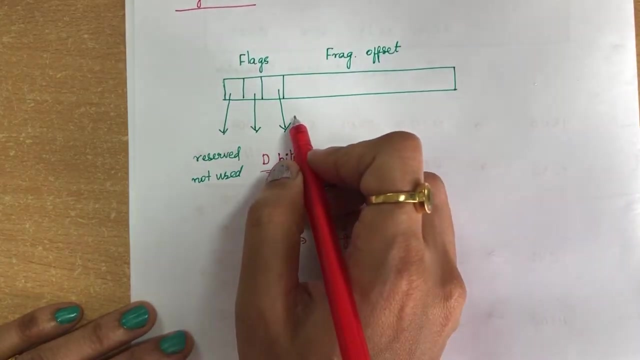 so, whenever the data, if it is the datagram it passes to the next router, if it wants the data, the router can fragment the data and it is purpose of the. it is the duty of the receiver to do all the reassembling of all the fragments at last. okay, the next last bit is called m bit. 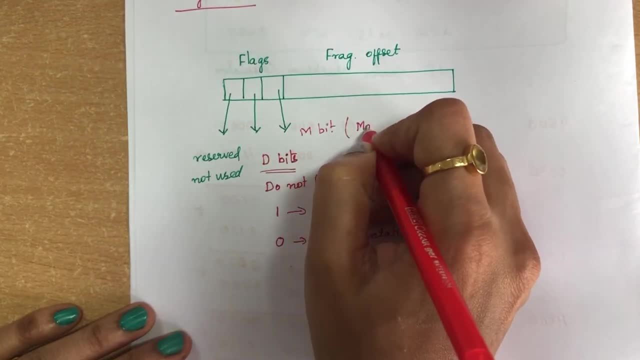 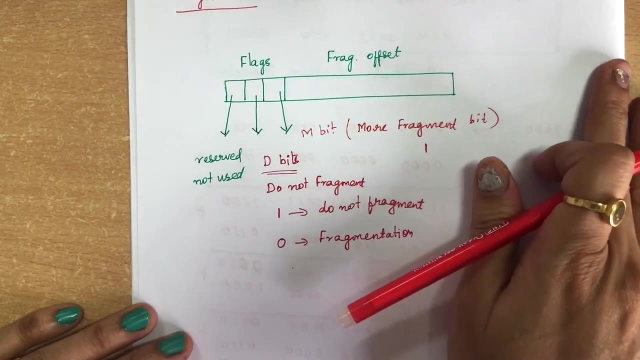 okay, the last bit is m bit. what do you mean by m bit? is m bit is nothing but more fragment? okay, more fragment bit. so when this bit is set to 1, when this bit is set to 1, that means: 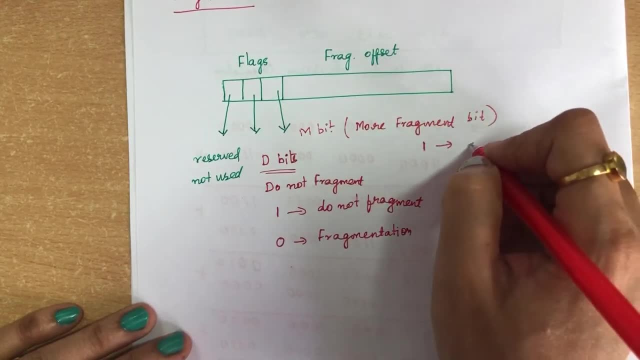 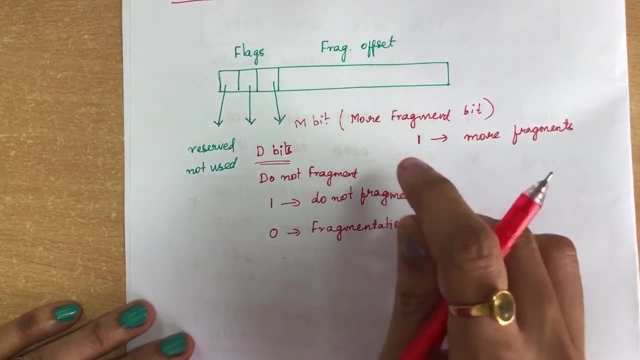 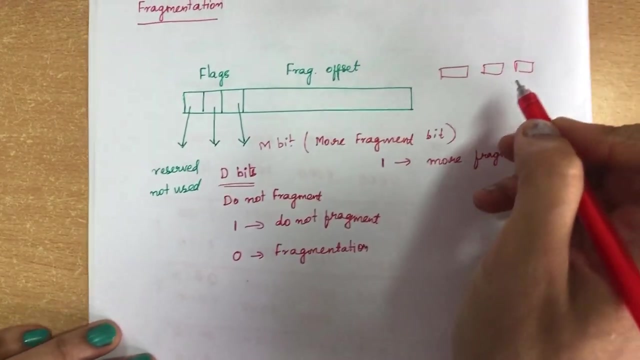 datagram. it is not the last fragment you have still more fragments are available. so when you are sending the data, sending the datagram, you will be setting this value as 1, if suppose, if you have fragmented and you have sent, so you have fragmented the data into 3 fragments and you are sending the 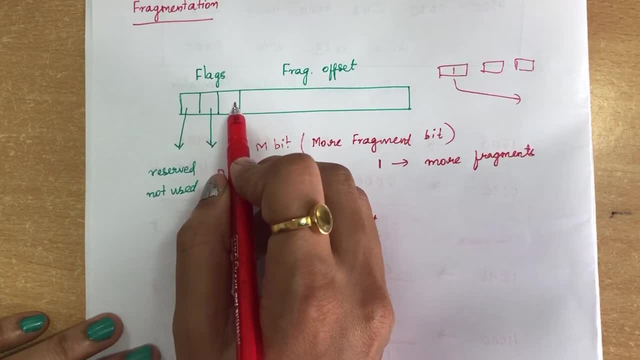 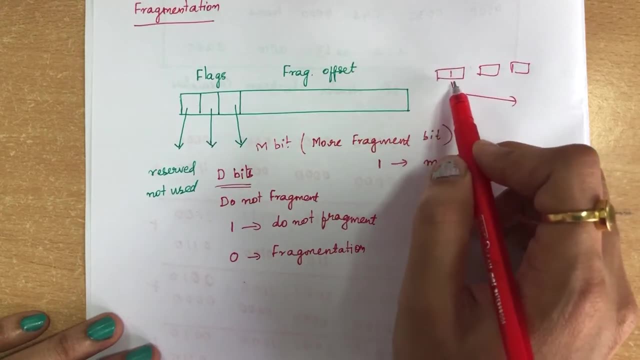 first fragment and in that you will be sending this value to be 1, that means still more fragments are there. okay, so the receiver will think that, okay, the data is not. it is not the last fragment. still some more fragments are there. when this value is set to 0, it means that this is the last. 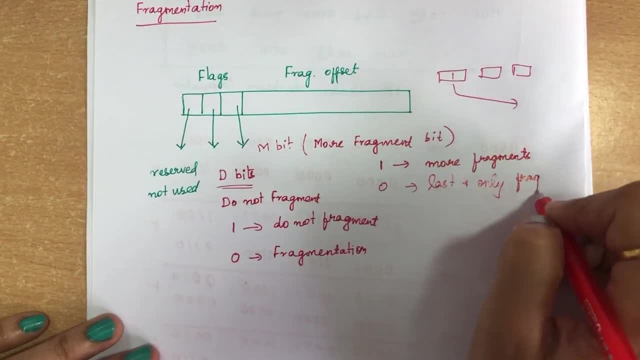 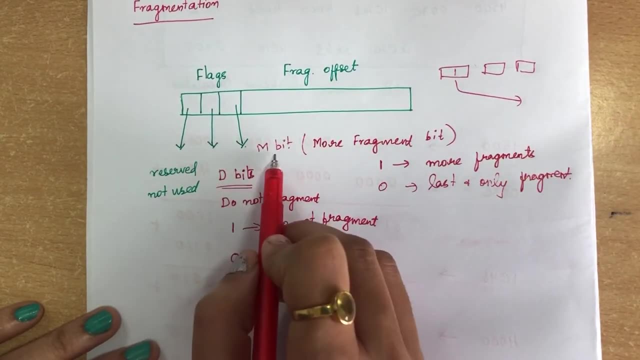 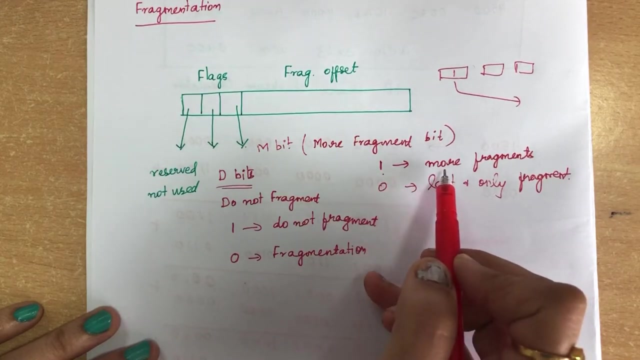 and only fragment. this is the last fragment, so after this, there is no data is going to come. okay, this is what this bit is going to mention you, whether you have more fragments or this is the last fragment. when this bit is 1, it means it is more fragment is there after this data, and if this is 0, this is. 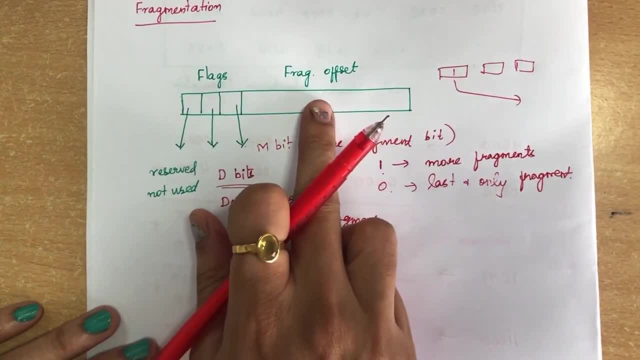 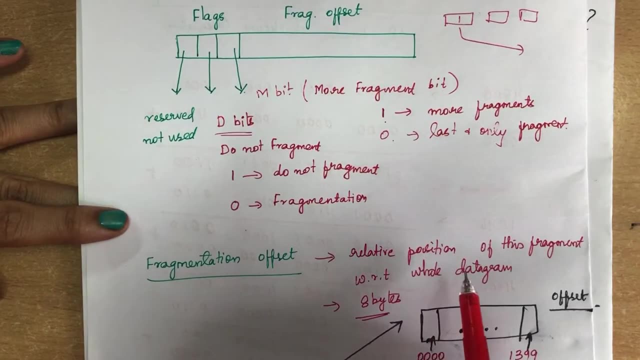 the last fragment. okay, this is all about the flags. Next we will see what is fragmentation offset. it is just fragmentation offset. the fragmentation offset value will tell you the relative position of the fragment with respect to the whole datagram. so this, you can say that. 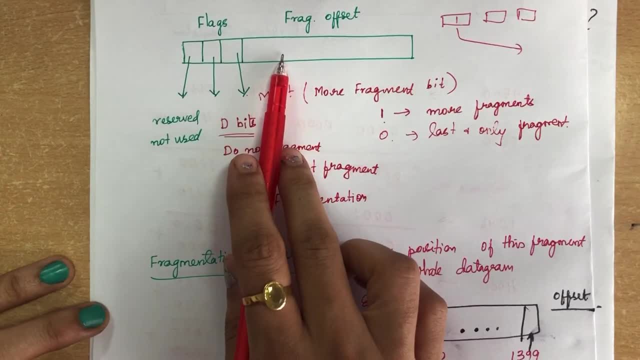 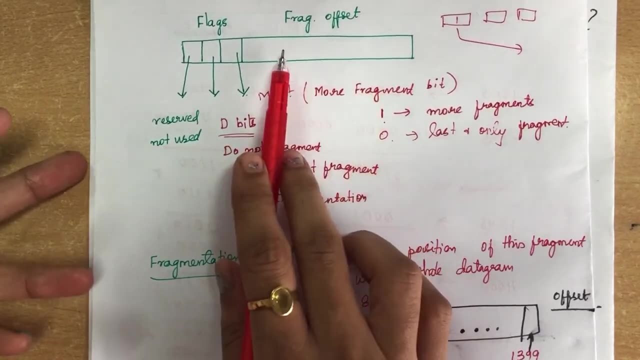 it is an offset of the data, so usually the offset of the data, since we cannot able to give all the values in the fragmentation, so we can give the offset values in this. so this is usually measured in 8 bytes. okay, so now we will see how fragmentation is done. 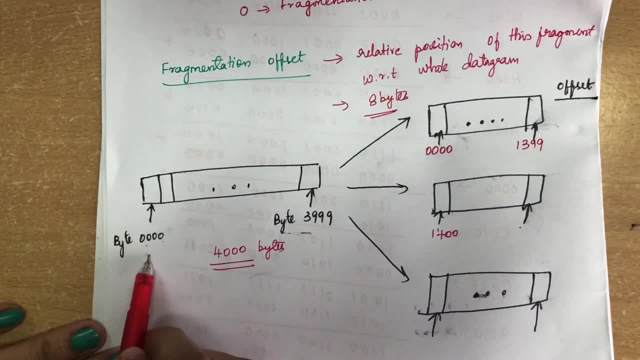 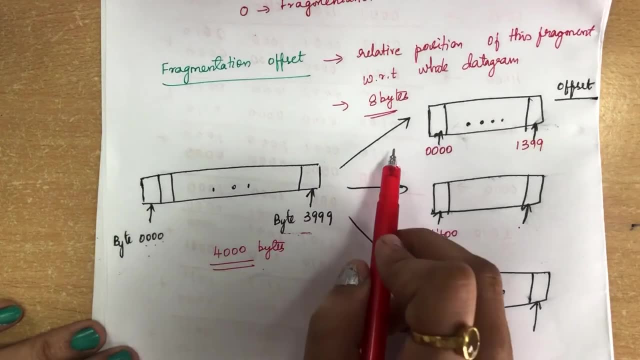 so you can see this. this is an original datagram. you have the, which consists of 4000 bytes of data, 00, starting from 000 to 4000 bytes. so now we are going to do into 3 fragmentation 3 datagrams. so which is which? 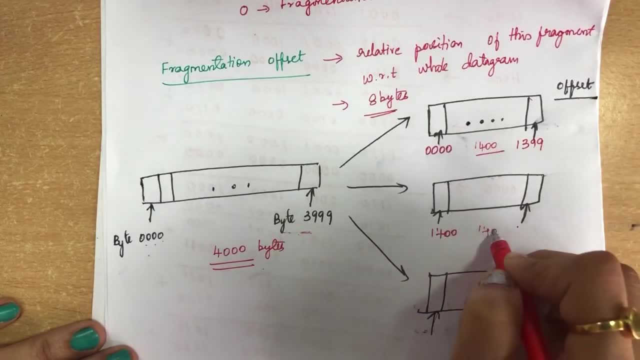 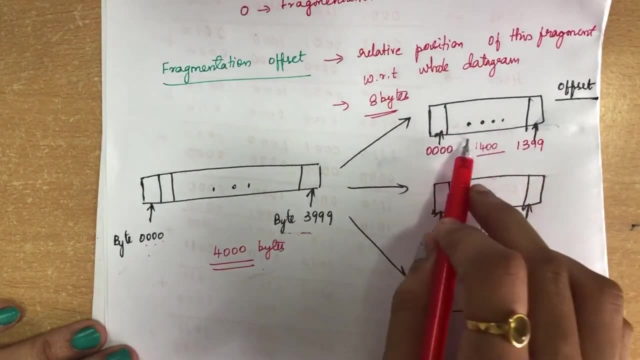 each containing 1400 bytes. okay, 1400 bytes and the remaining over. here we are going to have 1200 bytes, so, starting from 000 to 1399, we are going to do 1 datagram, another 1400 to next is 2799. 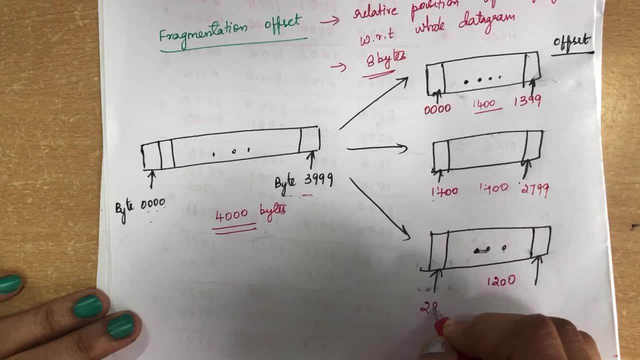 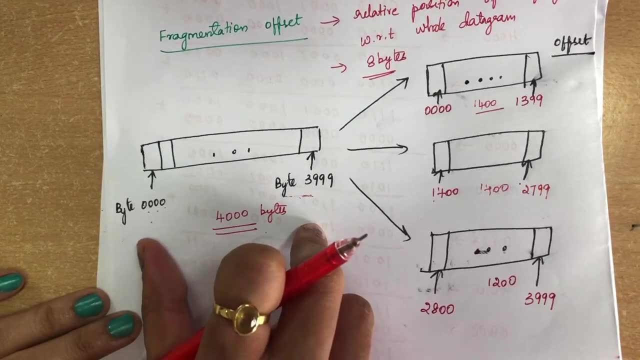 we are going to give other datagrams. And third one is 2800 to 3999. we are going to give the next fragmentation. okay, we are dividing the entire data, whole datagram, into 3 fragments, like this: first 2 containing 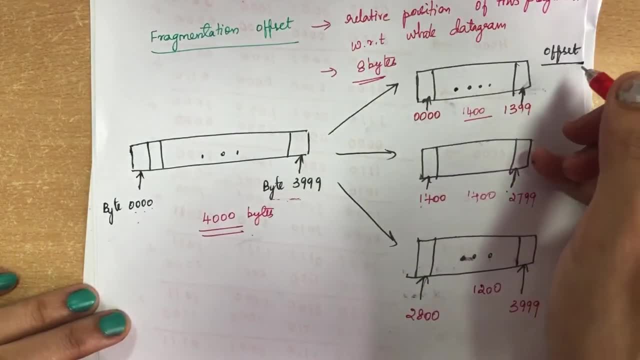 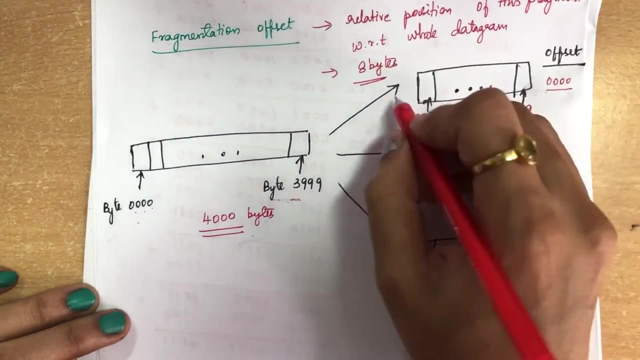 1400 bytes and the next one containing 1200 bytes. so now we will see how we will mention the offset value. so, since it is, I have told you like, it is measured in 8 bytes. so we have to take the first value, that divided by 8, that is nothing but 0, so the offset 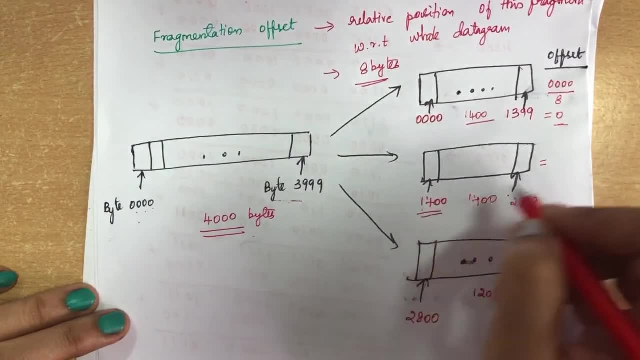 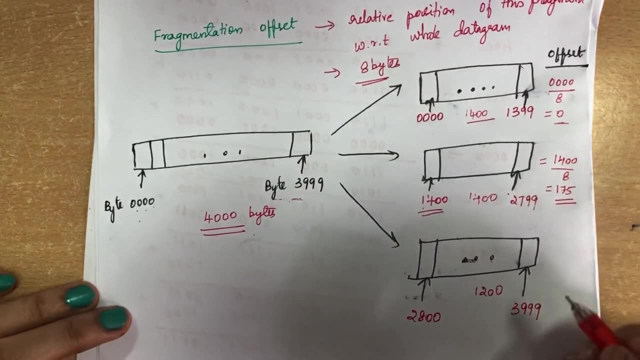 value for this is 0, so we have to take the first value. that divided by 8, that is nothing but 0, so this datagram is 0, and for this the starting value- starting byte value- is 1400, that divided by 8, we will get 175, so the offset value is 175. that will be mentioned. 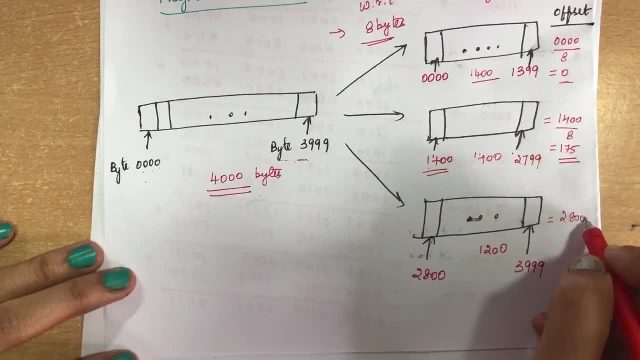 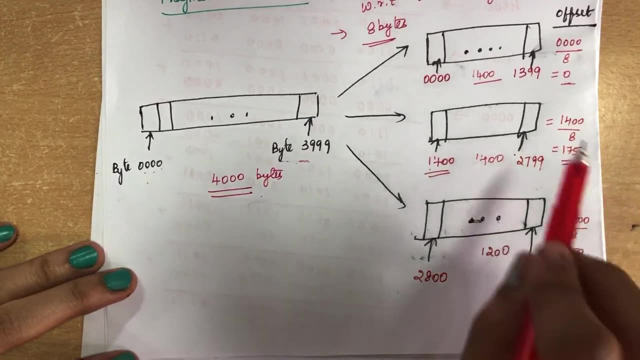 in that offset. So here the starting is 2800, 2800 by 8 that we will get 350, this is the offset. so this is how we will calculate the offset value, and these values are have to be added in. 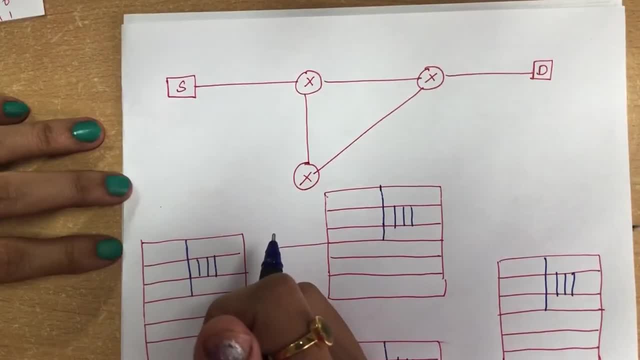 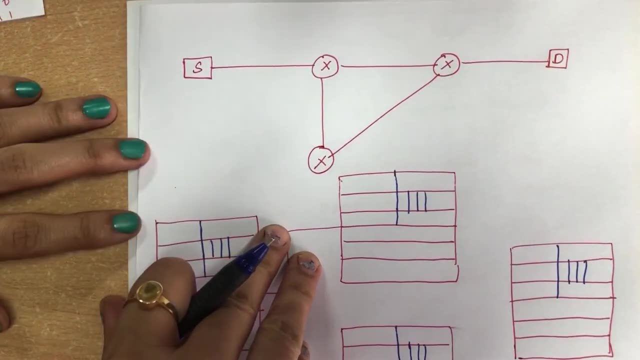 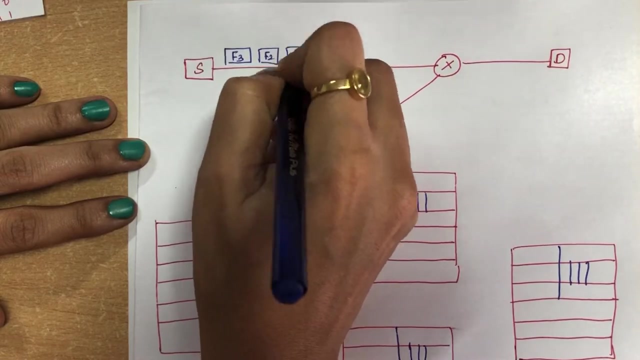 this offset, fragmentation offset. okay, So see a detailed fragmentation: how fragmentation works, works. so, for example, the data, which is which we have seen in the previous example, where we are dividing the data into three fragments. so initially we are dividing into f3, f2 and f1. okay, so we are. 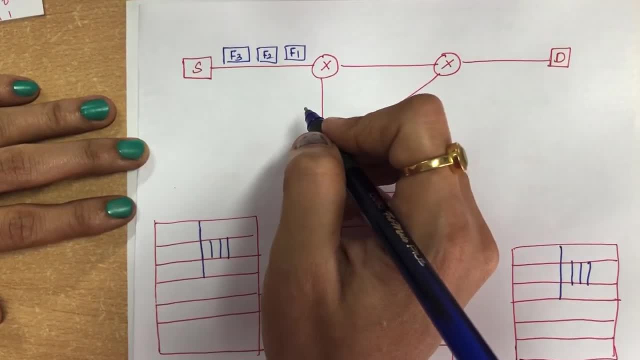 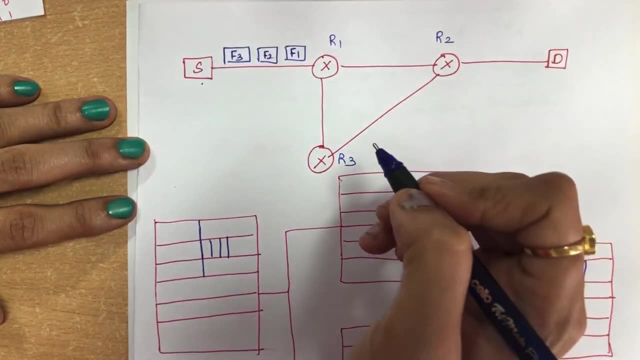 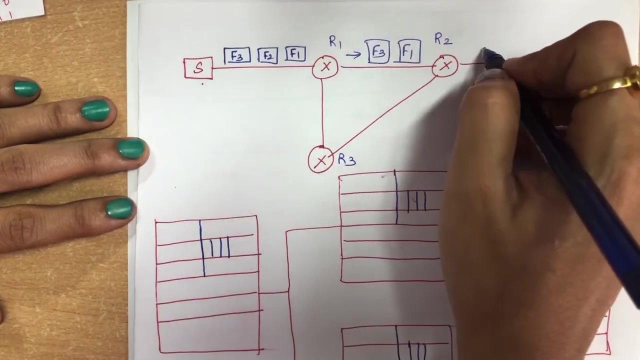 dividing into three fragments and we will see how reassembling is done in the destination site, so source site, and you have two routers in between, r1 and r2, and you have three r3 and here you have the destination. so this f1, so f3 and f1 will pass in this way through the router r1 and r2. 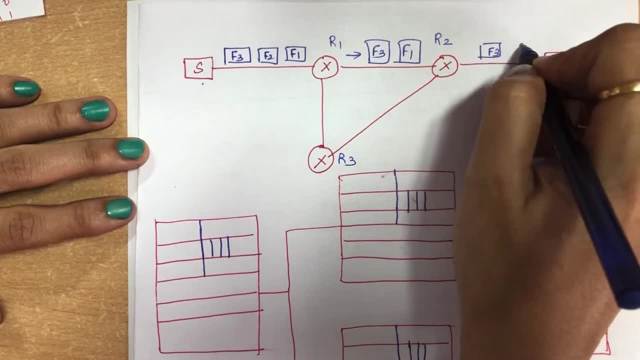 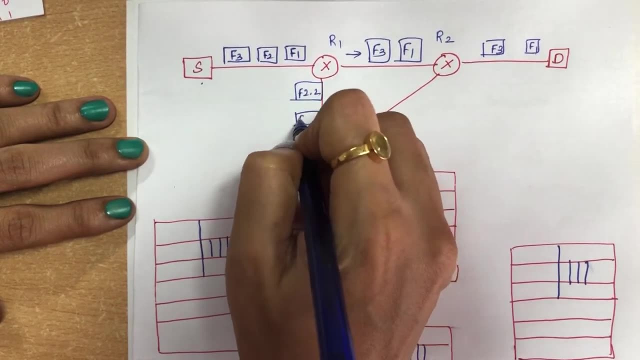 it will reaches your destination like this: f3 and f1- okay, but f2- it again divided into two fragments- f 2.2 and f 2.1- okay, and it reaches. it comes through the router r1 and r3 and again from r3. 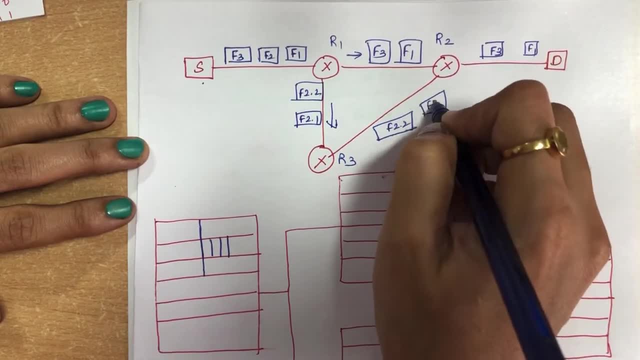 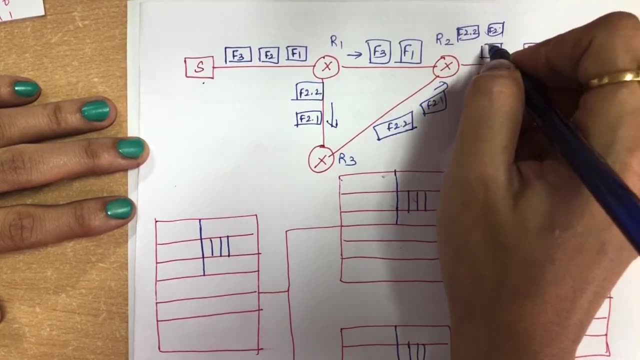 to r2, that is f 2.2 and here f 2.1. so at last, here it reaches, here f 2.1, f 2.2 and f 2.1. okay, likewise it goes on. so all the fragments will get reassembled over here in. 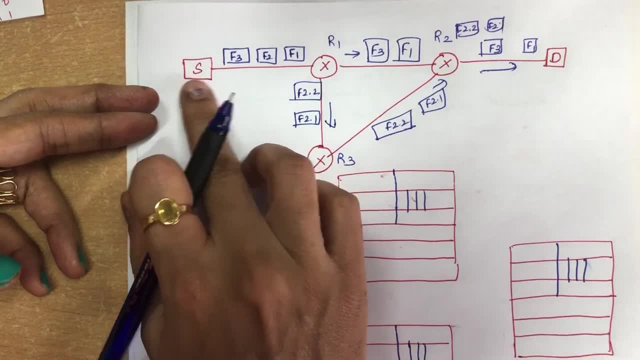 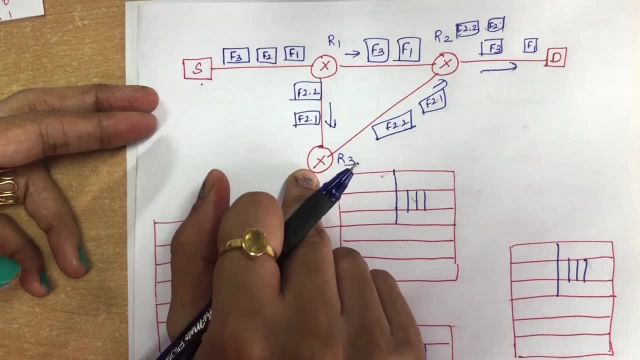 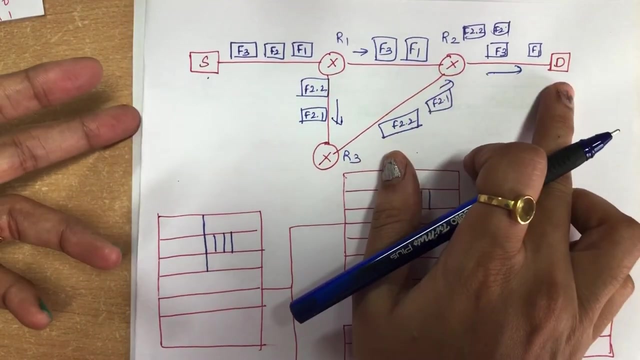 destination site. okay, so we are dividing the entire data. the whole datagram is divided into three fragments: f3, f2 and f1. it reaches router r1 and f2. it goes through the router r3 again. this f2 is divided into f 2.2 and f 2.1, and from here it goes to the router r2 and then reaches. 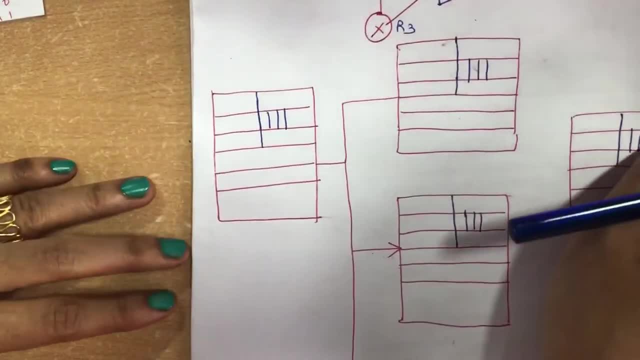 destination, but other fragments it passes through the same way. okay, now we will see how fragment termination work is done in the destination site. so we are dividing the entire data, the whole datagram. When fragmentation is done, how header will also header format also. it should be changed. 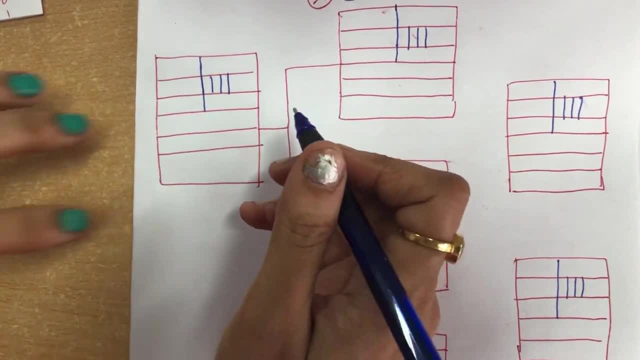 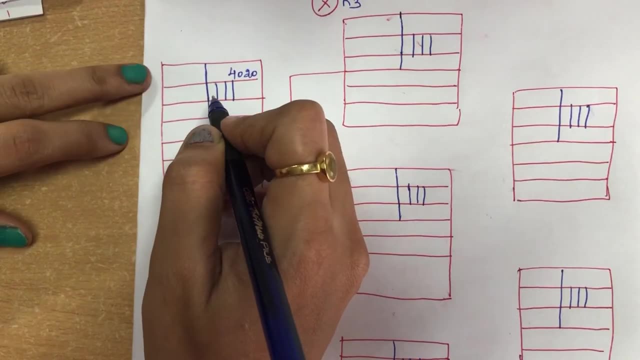 we will see that how it happens. So first over here, since it is 4000 bytes, so we will take in 4020 bytes over here, since in the it should be in the multiples of 8, we have taken 4020 and some identification. 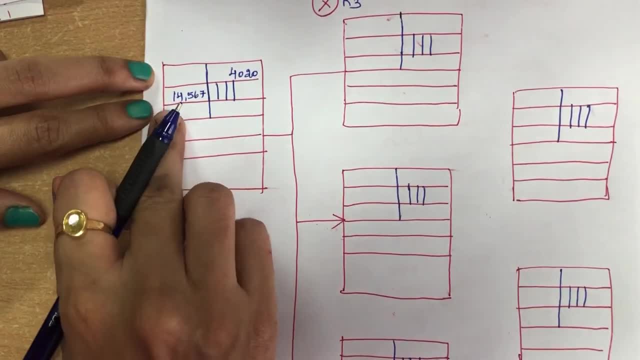 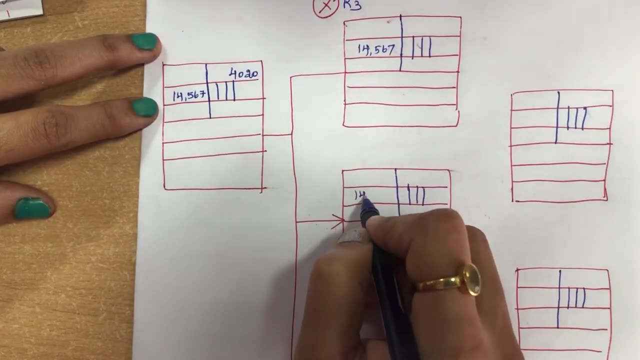 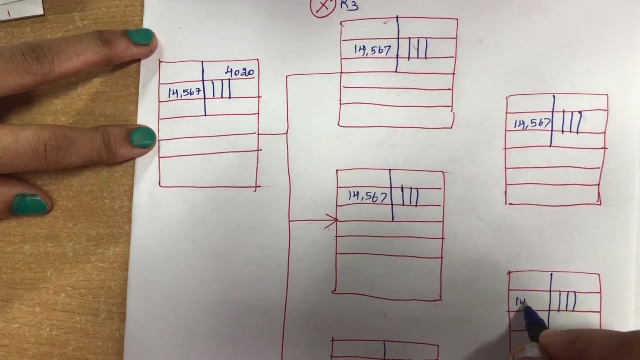 number should be given for every, all the fragments. so the data it is. we have given the identification number to be 14567, so which we will mention in all the sub fragments also 14567.. So it means that all the data it belongs to: the same data, same datagram. ok, 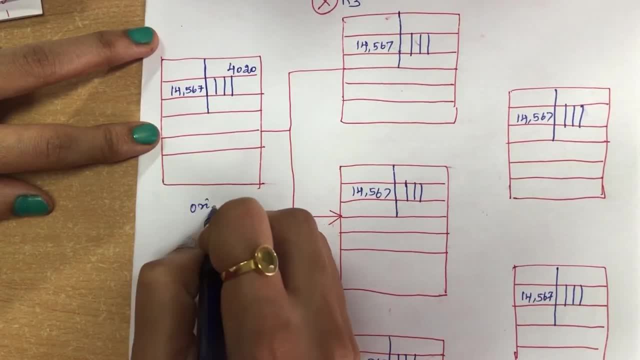 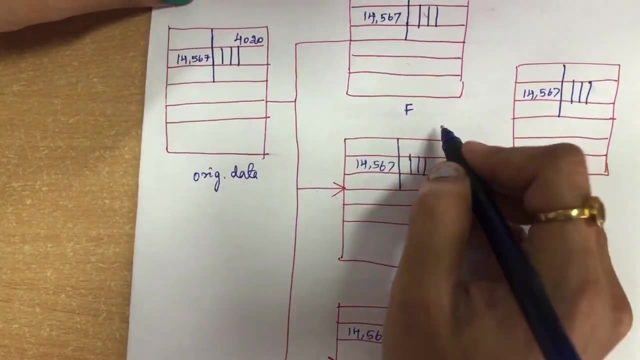 So here we are dividing the entire. that is original data. this is the original datagram and we are dividing into 3 fragments over here we have divided into 3 fragments. so F1, F2, F3. so this is the header format for the F1 and this is F2.. 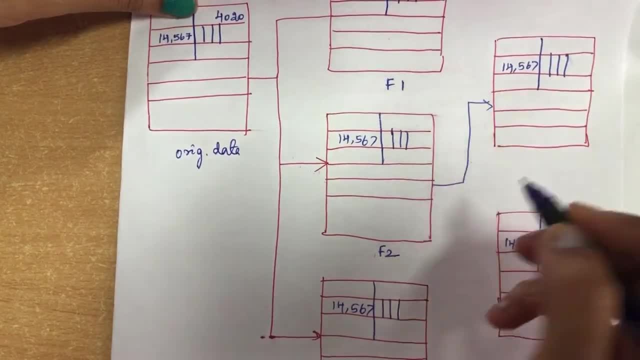 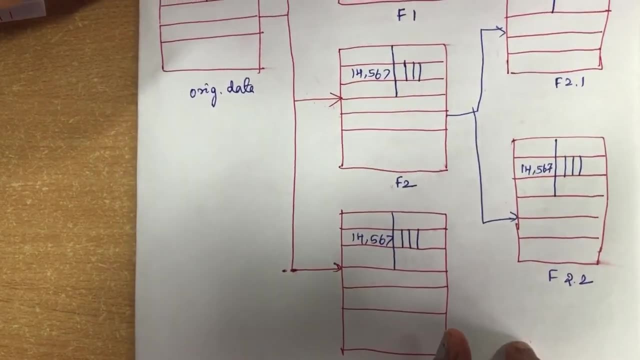 And F3.. Ok again, this F2 is subdivided into 2 fragments. that is F2.1 and this is F2.2. ok, F2.1 and F2.2. so whenever fragmentation is done, separate header will also be added to each datagram. 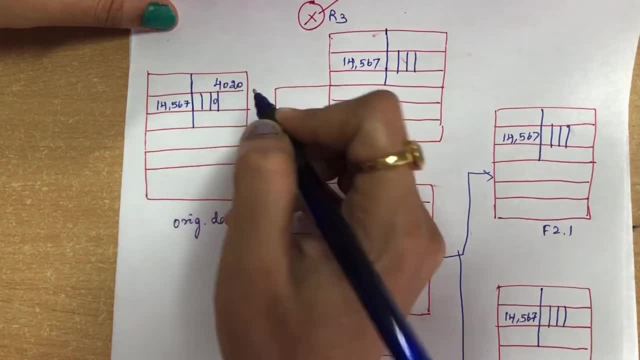 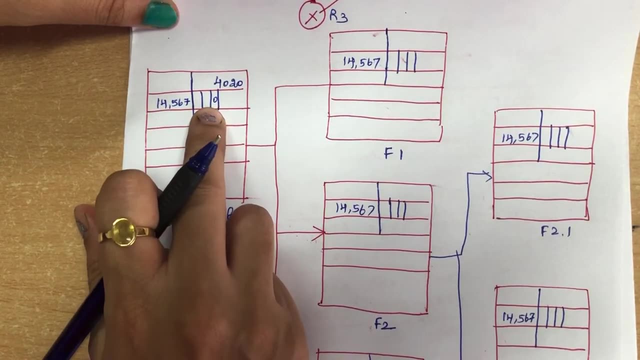 ok, So now we will here the m bit. m bit over here is 0. since there is no fragment for this particular original datagram, we are giving this m bit to be 0 and the offset value is 0. ok, the offset is over here. 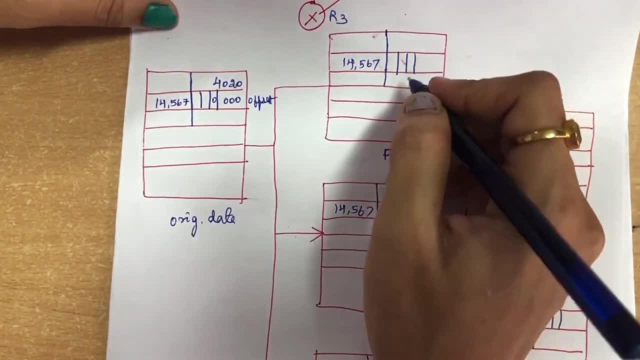 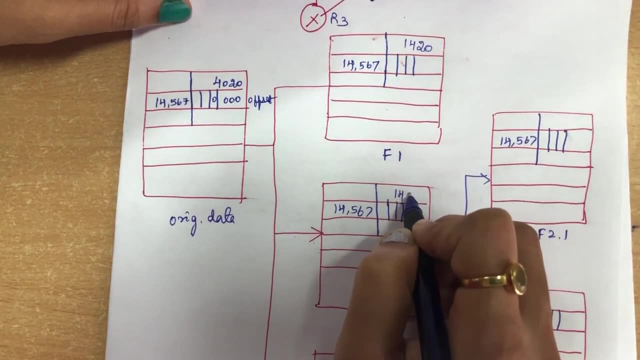 So it is 0 0 0. when coming to the first fragment, here it is. we are going to mention that, since it is divided into 1400 bytes, so each 1400, 1420, 1420 and the remaining 1220 is given to. 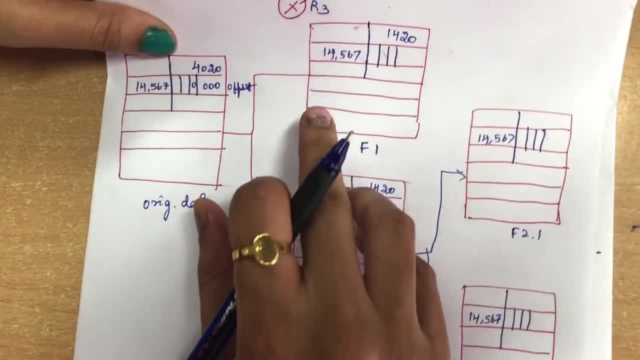 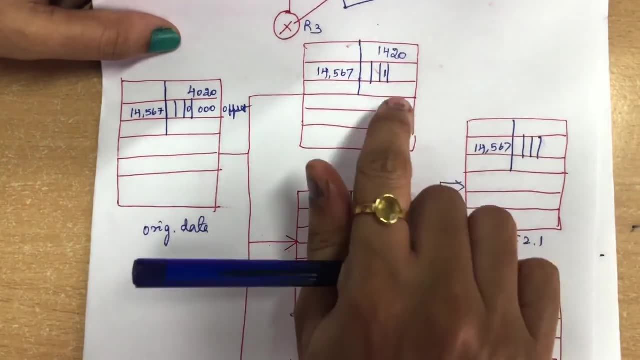 this particular near the last fragment, call F3. now we will mention what is the m bit over here. m bit over here is 1, 1 because still you have more fragments. so we are going to set the value m bit to be 1 over here, the flag bit to be 1.. 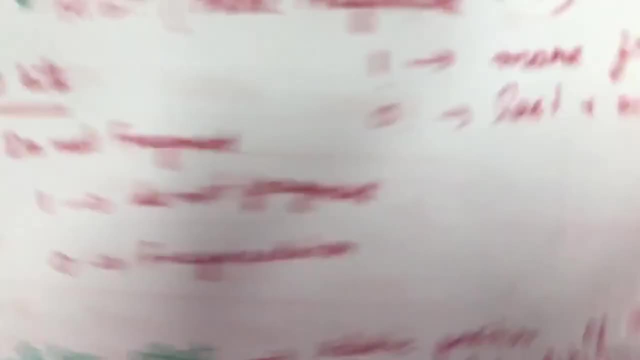 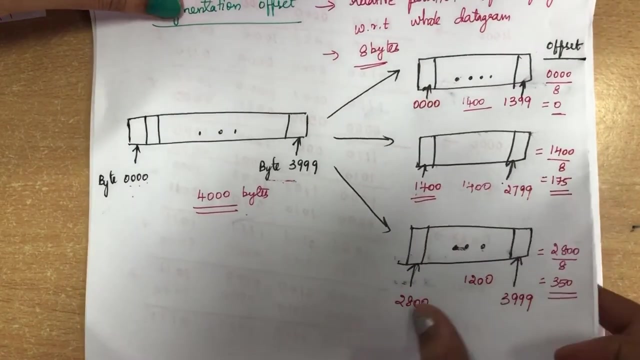 And the offset value, as I have told you in the previous case- offset value, how to calculate the offset value. the first fragment it is 0, the second fragment it is 175 and for the third fragment is 350. so that value you have to mention it over here. so the 0 0, 0 for the 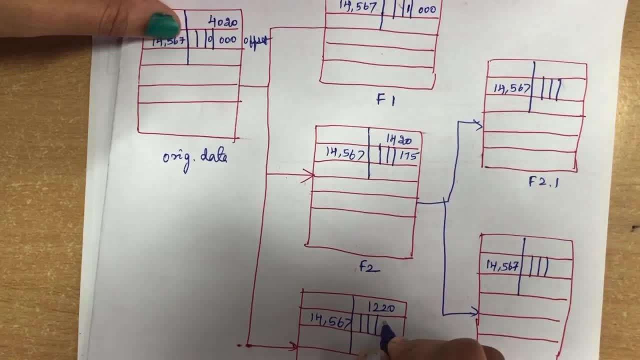 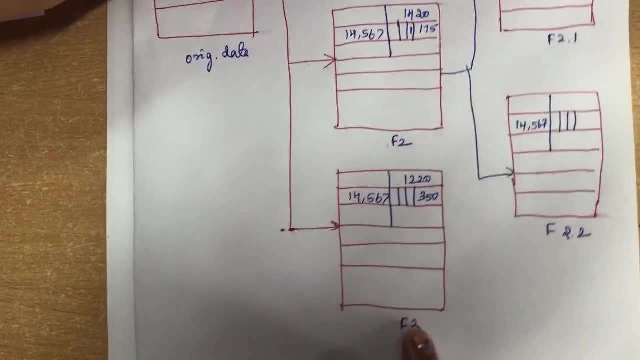 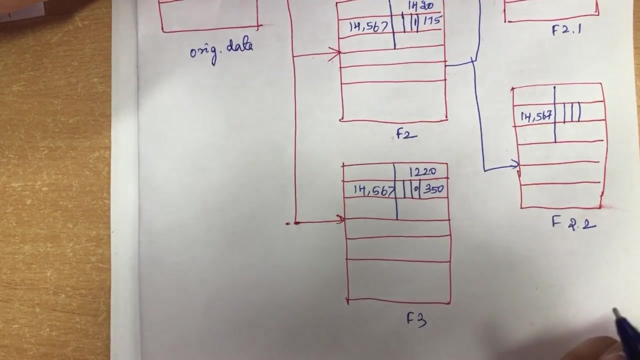 first fragment, second fragment, it is 175 and for the third fragment it is 350. ok, the m bit for this value is also 1. still, you have more fragments. but coming to the last fragment, F3. fragment next to it. so here the m bit value will be 0 over here.